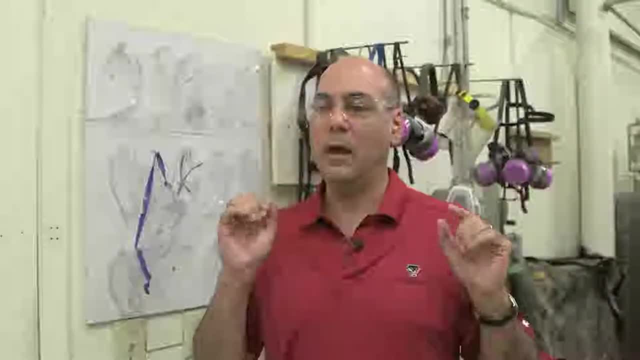 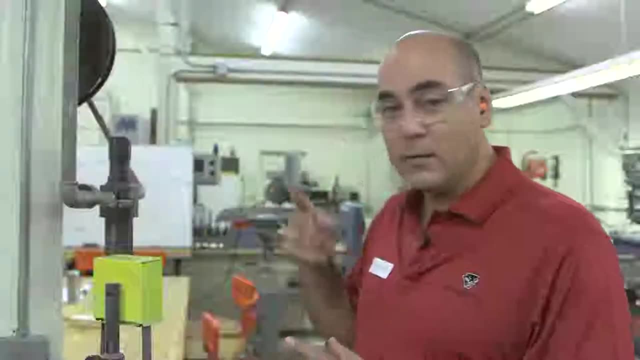 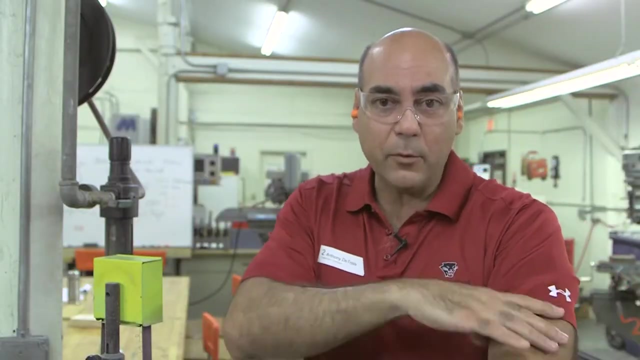 any questions again, just ask any of us Before operating any piece of equipment. equipment moves, spindles turn, our long hair is tied up, our sleeves are rolled up or tied. tight shirts tucked in, no big necklaces hanging out. safety is not a concern. We are here. 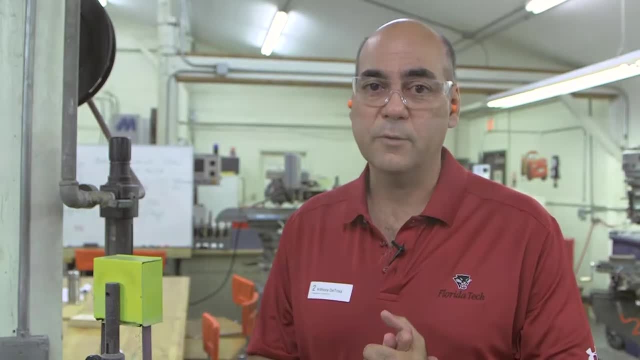 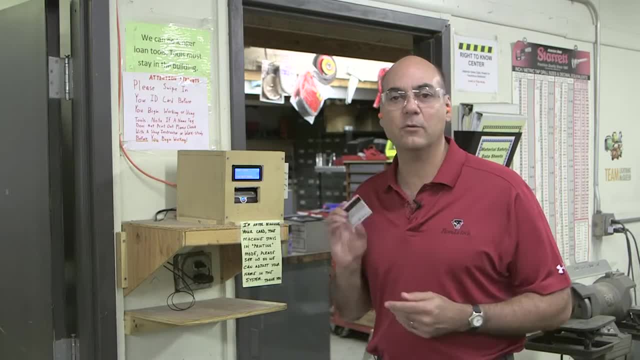 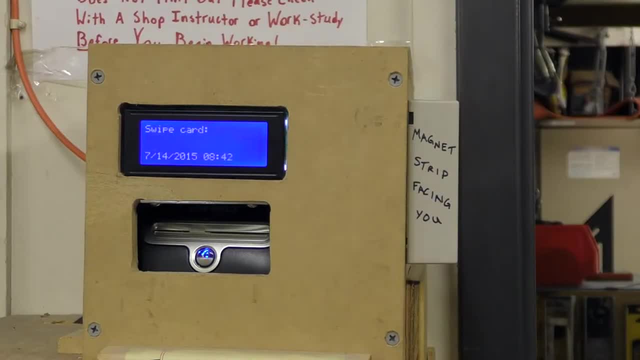 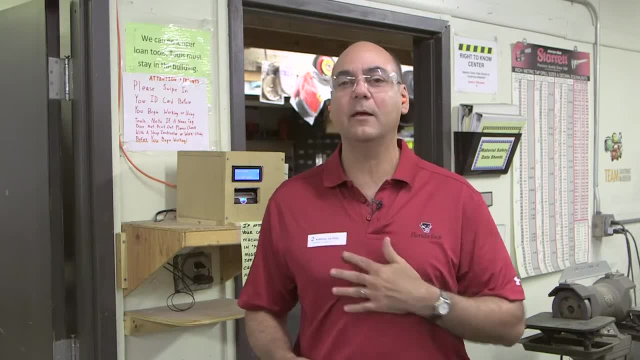 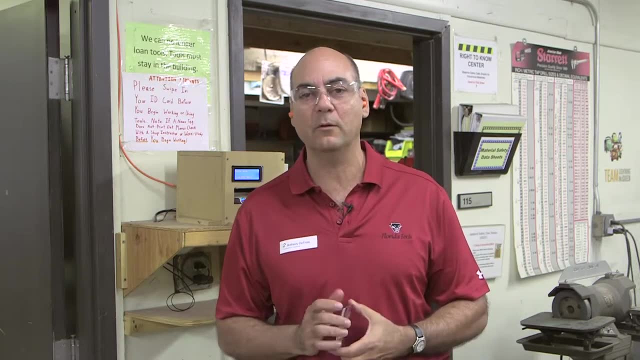 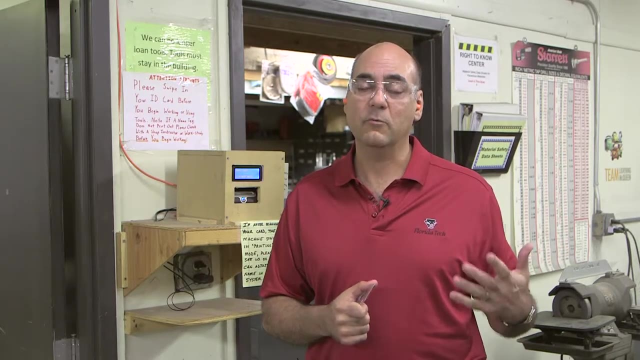 Your label has to be placed somewhere on your body that is visible to us. That way, when we scan the room, we look, see everybody's labels and we know that everyone's certified. That's operating equipment. If your certification is not current, you have to come see us and you'll sign up for a recertification class. 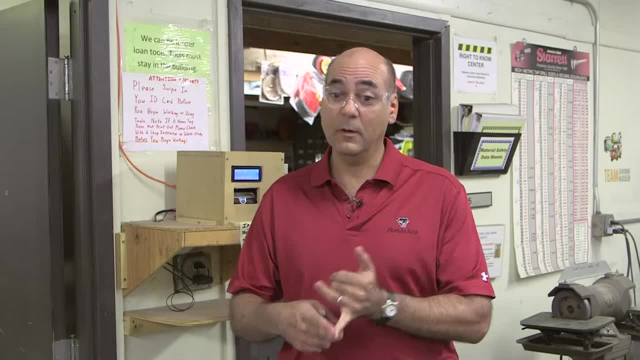 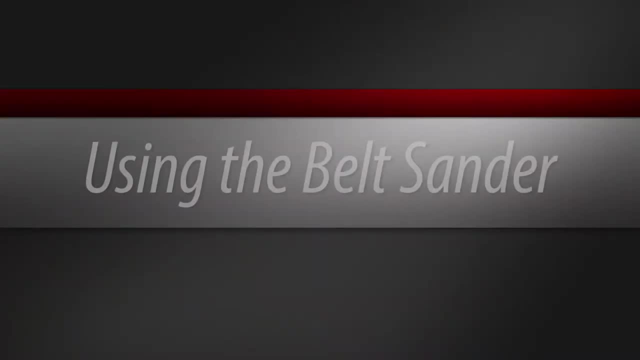 Recertification requires you watch a video, a safety video. We go over the shop rules and you take a test. Okay, here we are with the belt sander, The belt sander. we are going to deburr the part. 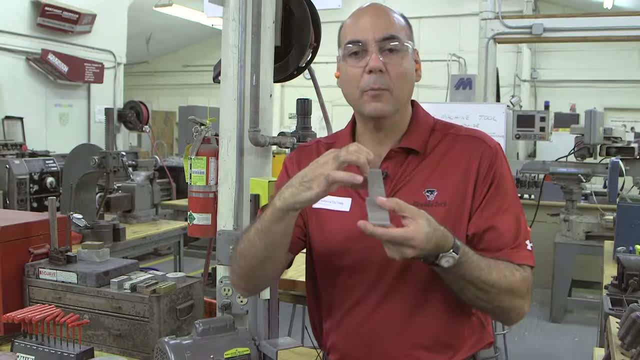 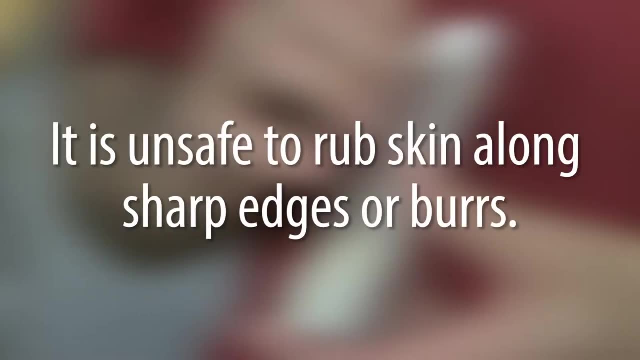 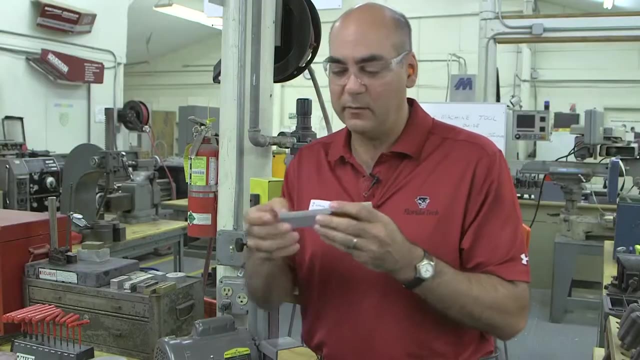 The part, this particular part was saw cut. There are sharp edges on it. I can feel them with my fingernail. My fingernail is catching First step. We want to get rid of the burrs, so we're going to come over to the belt sander. 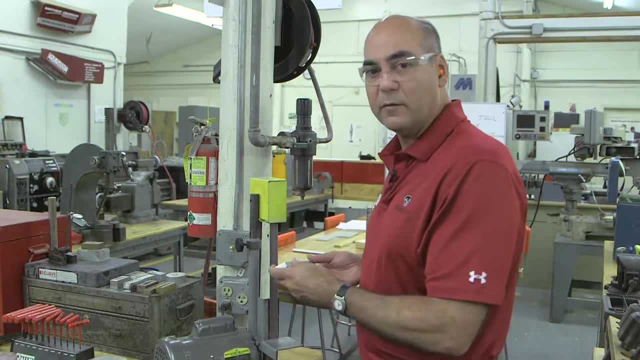 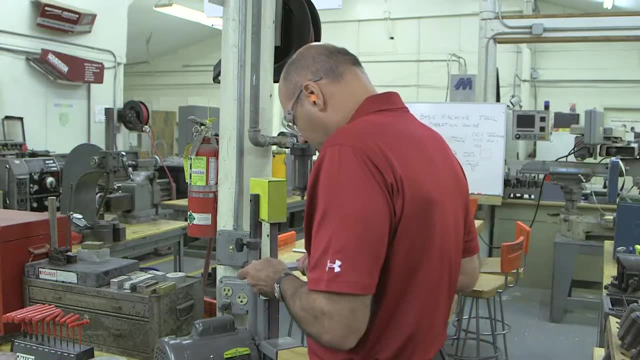 We are going to hold the part at approximately a 45-degree angle. get a good, firm grip on it and because the belt is not as wide as the part, we're going to have to travel the part back and forth to take the burr off. 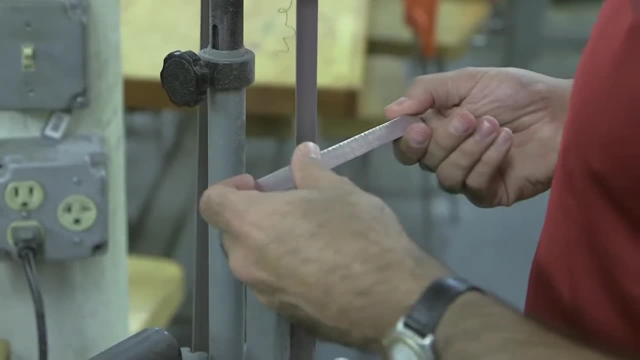 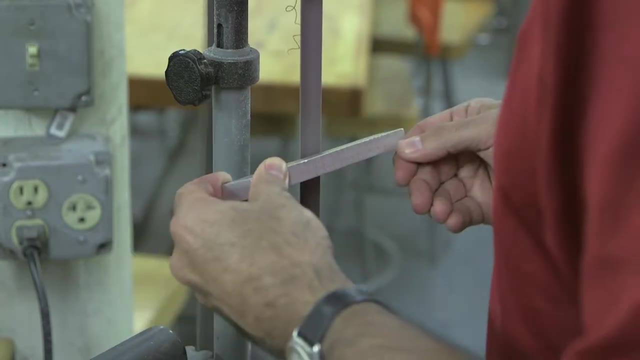 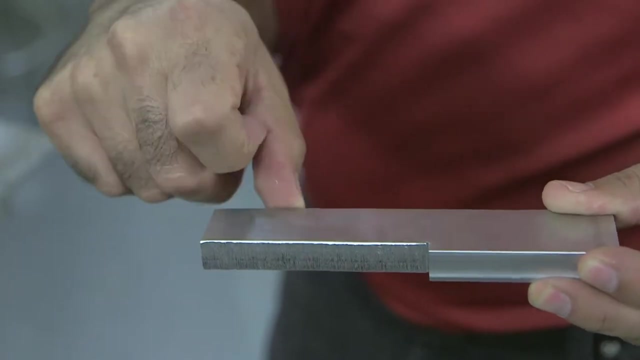 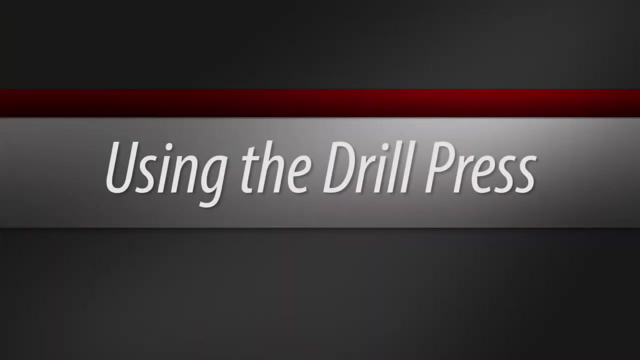 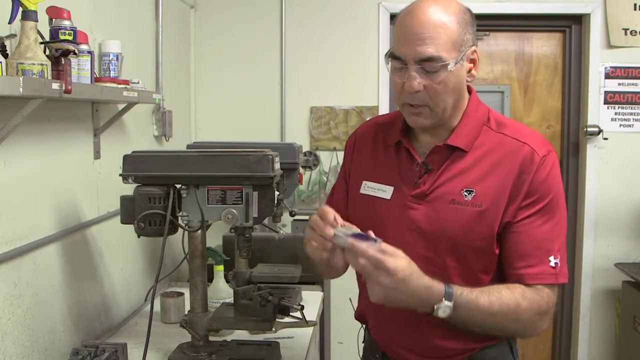 I am staying totally focused. The burr is gone. The burr is gone. Shut the machine off and then we're done. Okay, here we are with the drill press. Here is our part. It is already deburred. There's no burrs on it. 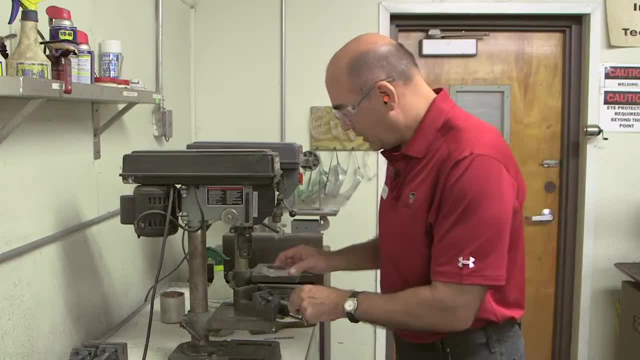 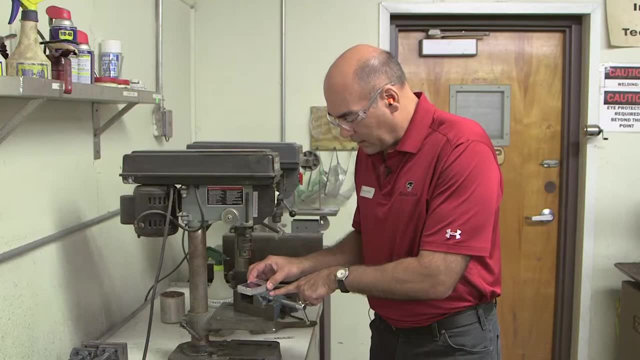 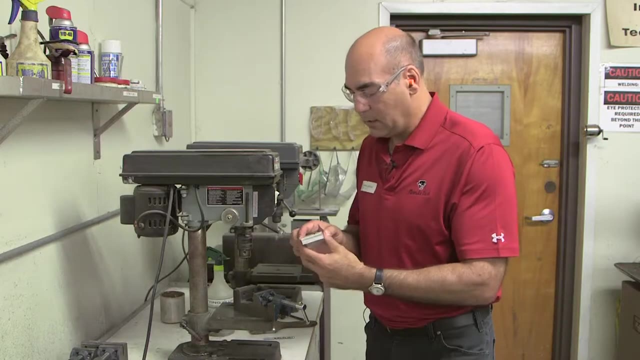 There's another reason why we want to make sure the part is deburred is so that the part sits properly in the work holding device. in this case we're using a vice. if there is a burr on it, exaggerated, the part is going to sit crooked and we're not going to be drilling a hole square to the top surface. okay, the other. 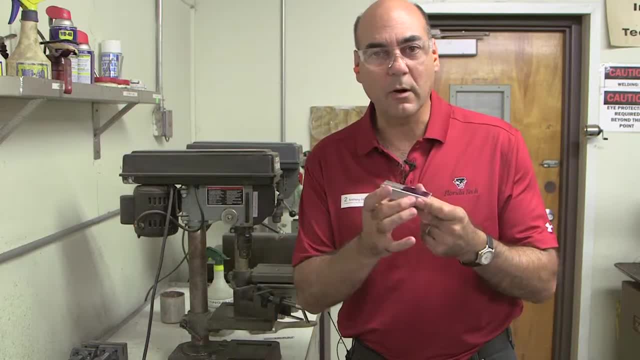 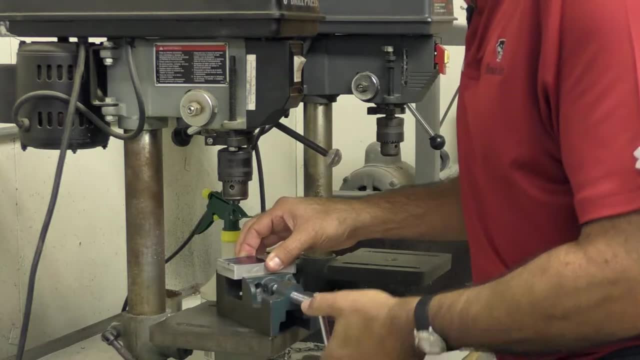 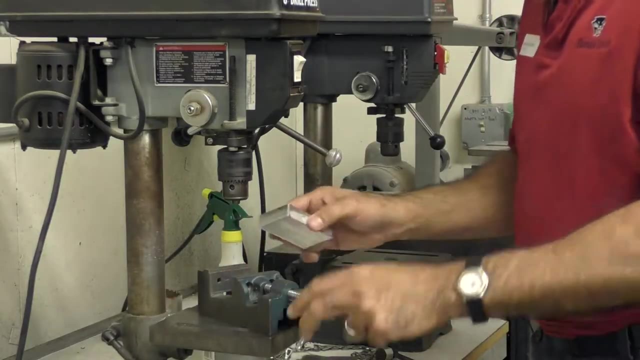 thing we have to pay attention to is that the sides of the part are parallel so that when it sits in the vise it's being squeezed properly. we are making sure that the vise is clear and clean of chips and that the table is clear of chips again, if there's chips, if it's sitting on chips. 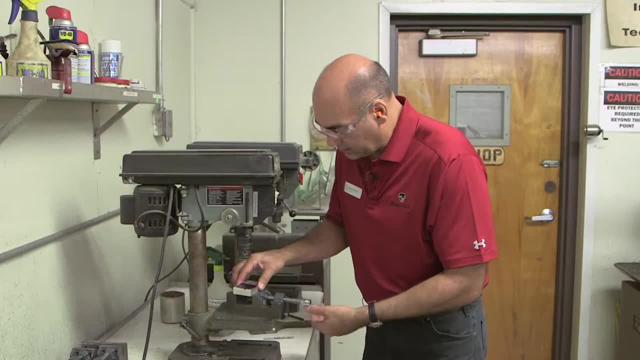 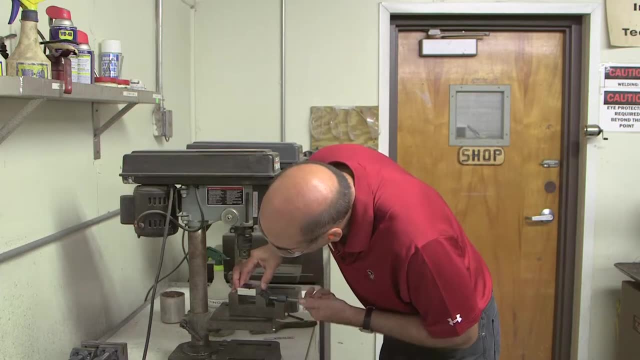 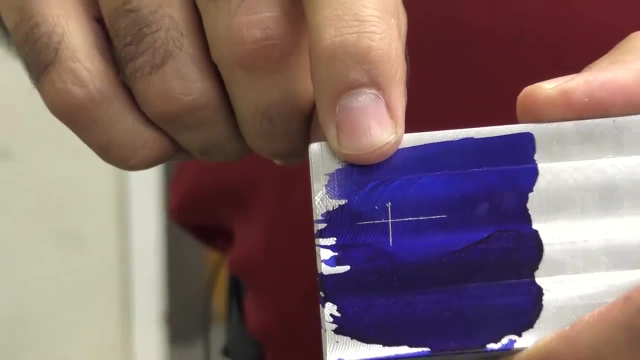 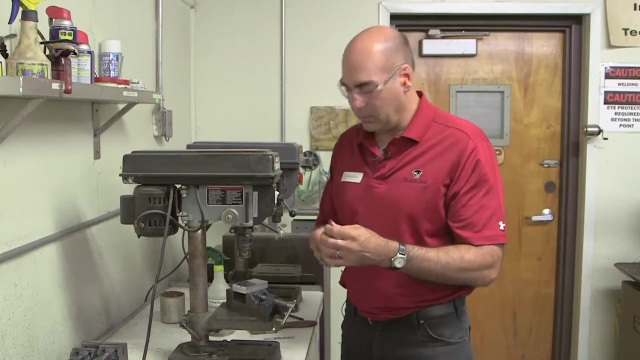 the part is going to sit crooked. okay, we put our part in the vise and we make it tight, tight. I have put on here, I scribed out, some crosshairs. that that's our point, where we need to drill our hole. the first thing we're going to do is we're going to drill with, we're going to spot the hole it creates a. 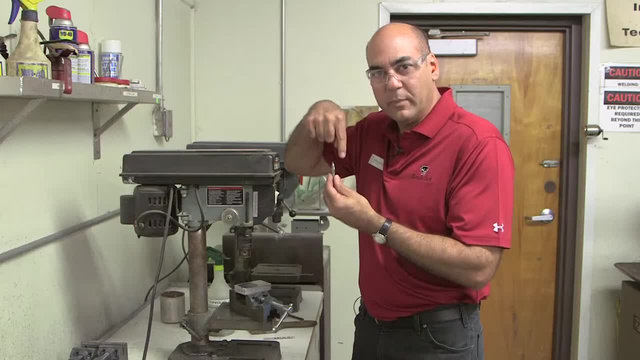 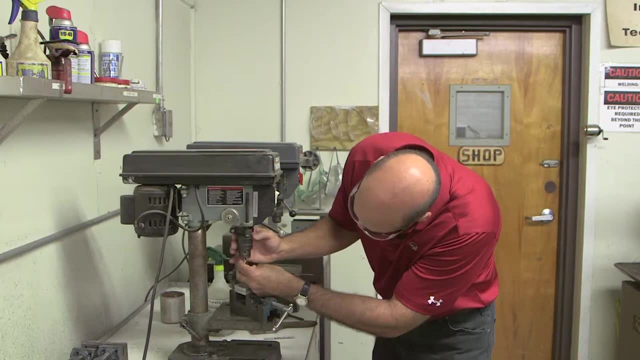 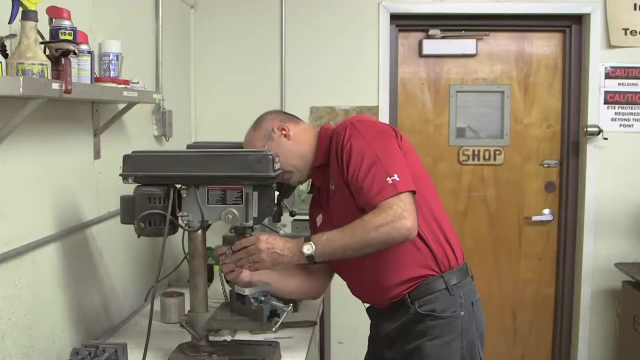 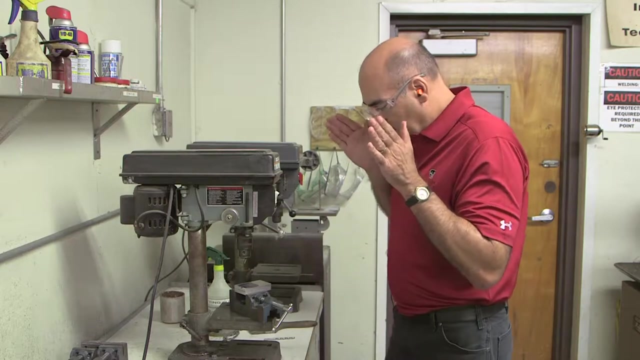 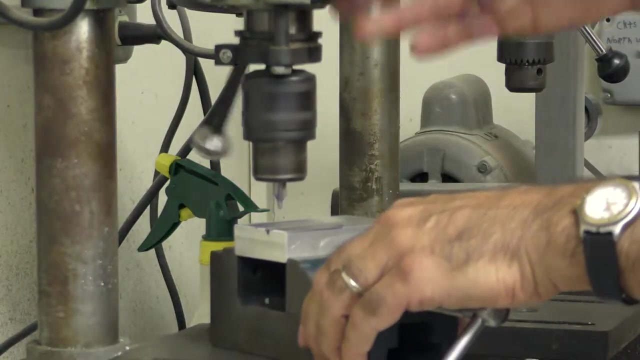 little location so that this drill bit doesn't wander. it follows the spot. we're using a center drill. right now we're loading the center drill into the chuck, tightening it with the chuck key, totally focused, not paying attention to anything else. okay, I want to line this point to the center drill up with the crosshairs. so I'm looking in. 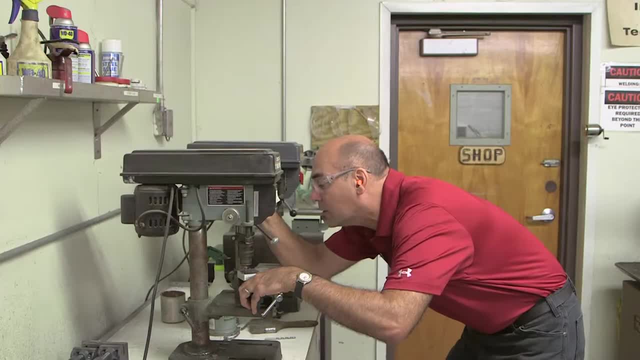 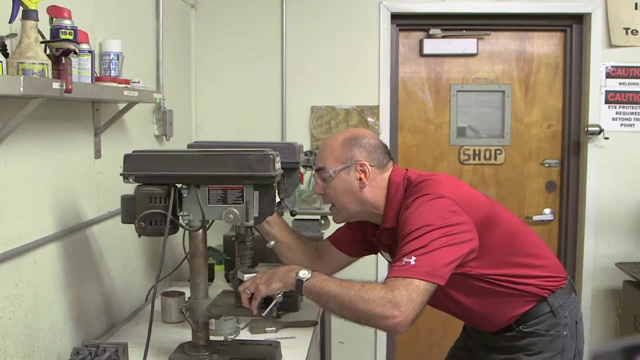 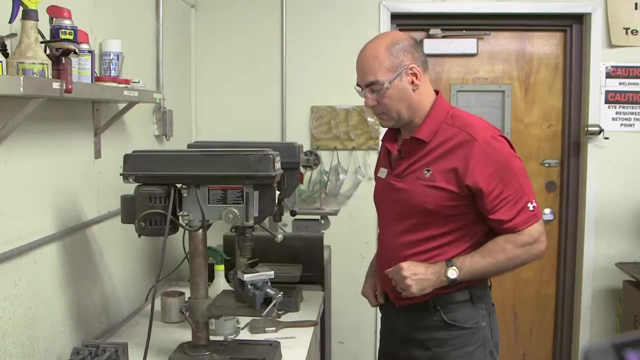 two directions. I'm going to look in this direction. make sure I'm lined up that way. and I'm going to look in this direction. make sure I'm lined up this way. once I peel them in the right spot, I'm going to Center drill the hole by. wait till the spindle stops before I clear any chips away. 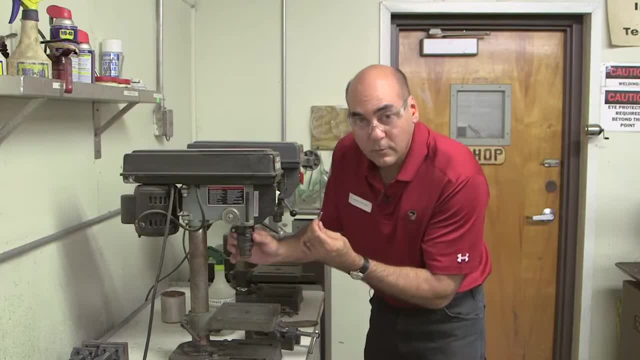 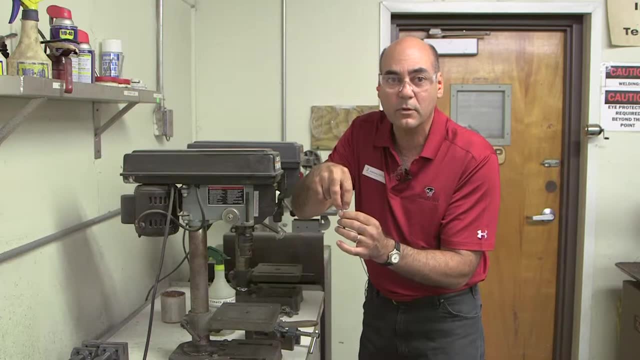 when loading the drill bit into the chuck- the three jaws that come out of the chuck- I want to make sure that the drill bit is in the center of the three jaws, that it's not in between two of them. if that's the case, the drill bit is going to wobble. 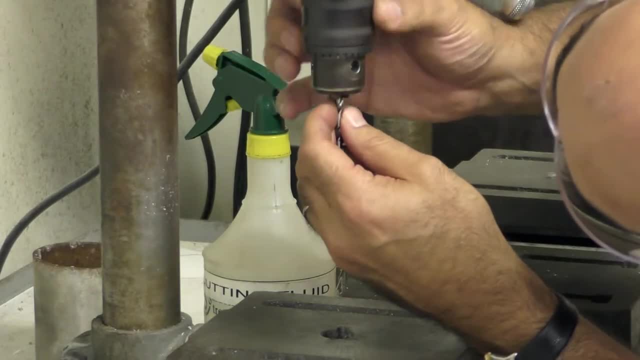 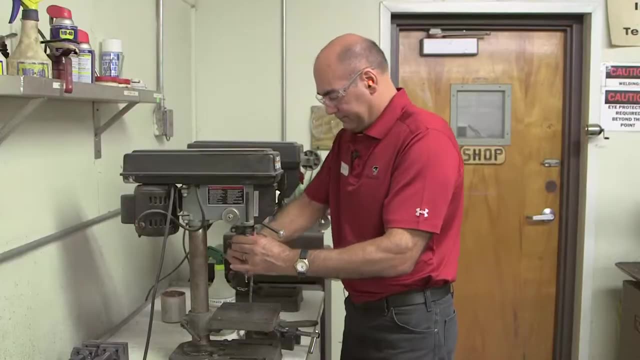 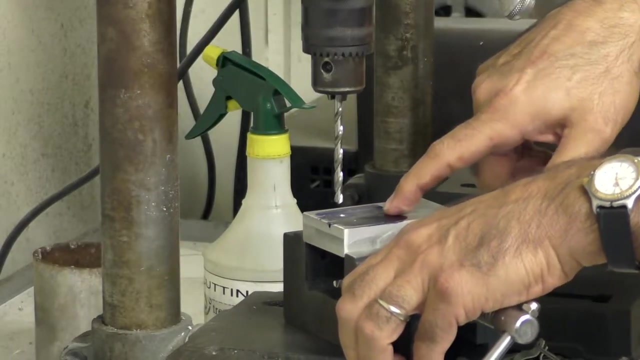 around. So I'm looking, making sure that the drill bit is centered to the three jaws and I tighten the chuck. We spotted the hole already, so the drill bit is going to start in the proper location. It's not going to wander off. 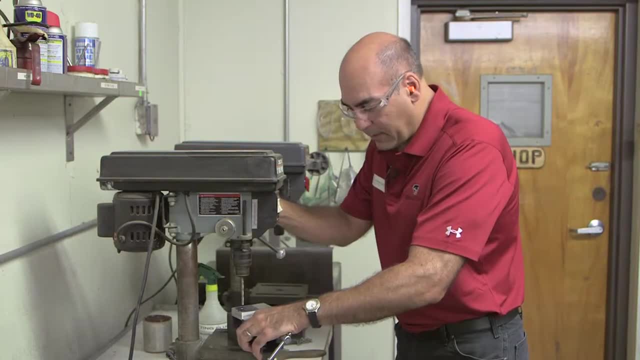 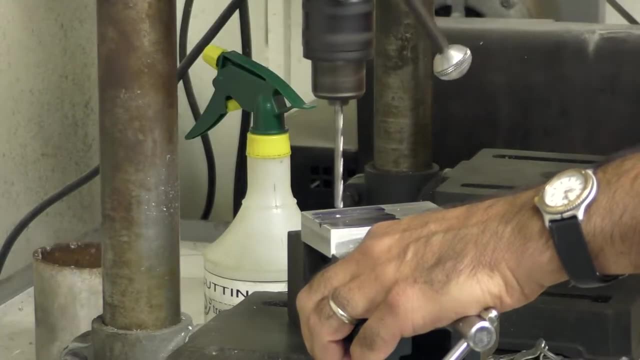 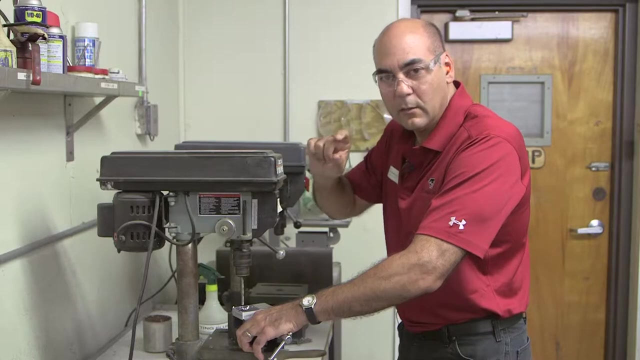 Turn the spindle on. I want to get a firm grip in my left hand, yet allowing it to center itself to the hole. Once it's there, I'm going to just commit and go. I am going to peck, drill, going to go approximately one-eighth down at a time. 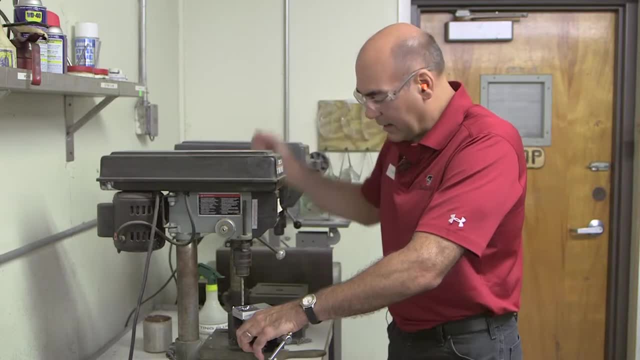 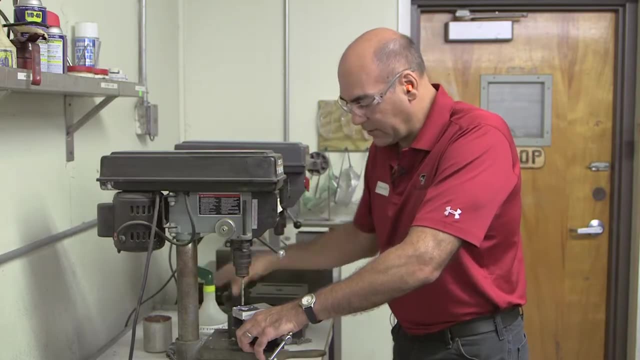 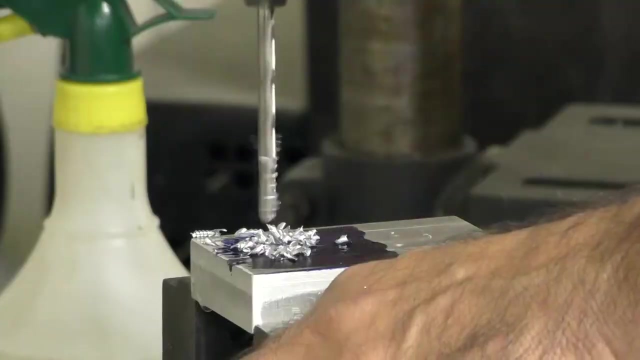 That way the chip breaks and I allow coolant to get back in the hole. We're using coolant: It cools, lubricates, It flushes the chips away. So I am peck drilling. Come all the way out and do another spritz of coolant. 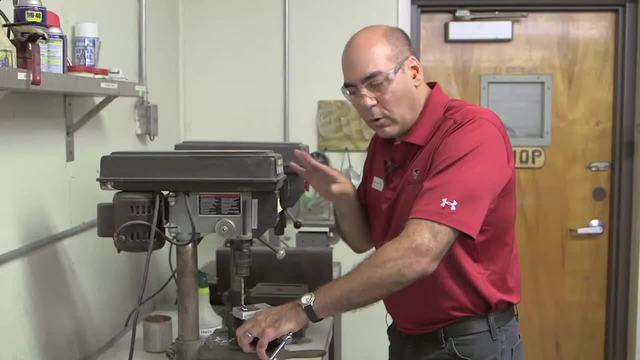 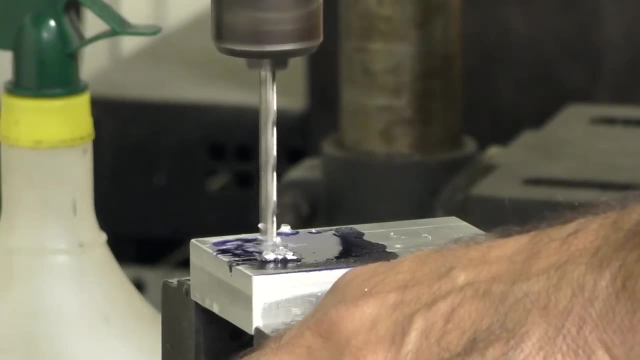 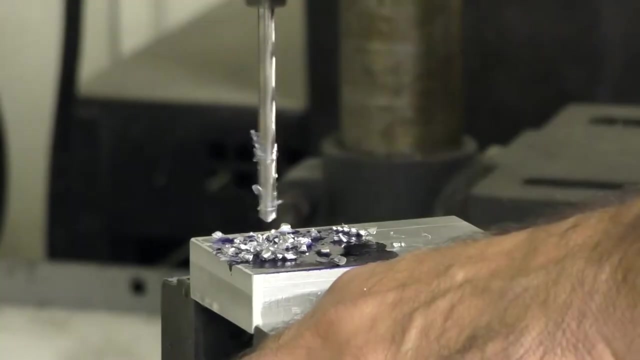 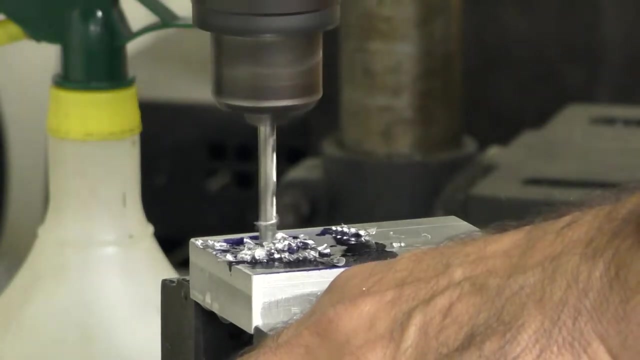 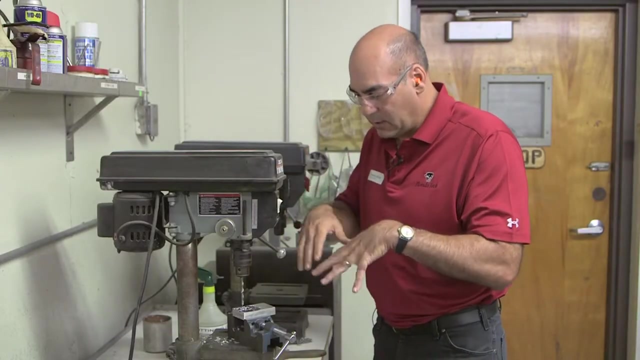 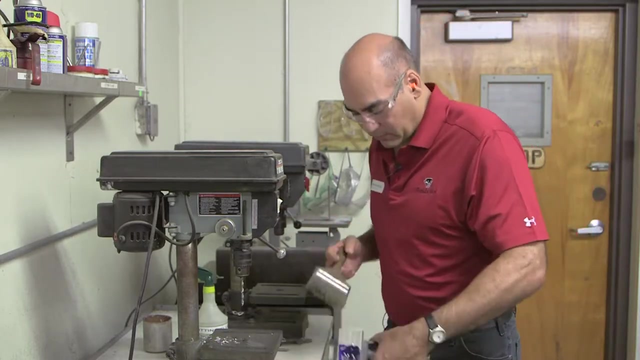 When you feel the drill bit starting to break through, you don't peck anymore. You continue all the way through, slow and steady. That's it. Good, firm grip as you're breaking through. so the part stays down on the table. The spindle stops before you clear anything away. 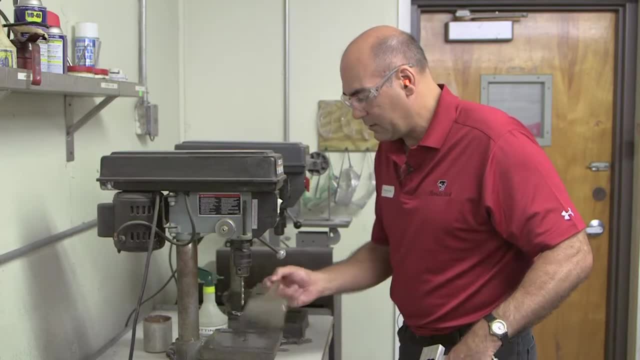 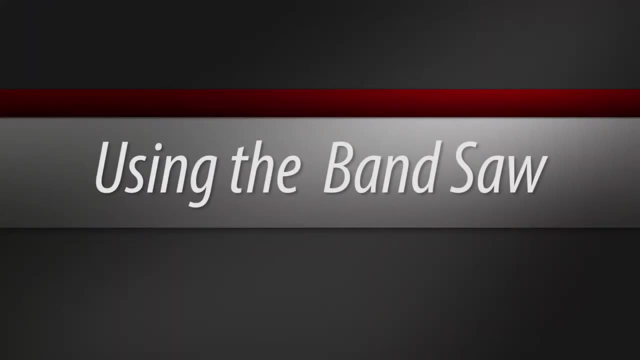 When you're all done, you take the brush, clean everything up for the next person. Okay, You should be ready to go. Thanks, See you next time, Bye, Bye, Okay, Now we're on the bandsaw Again. totally, totally focused. 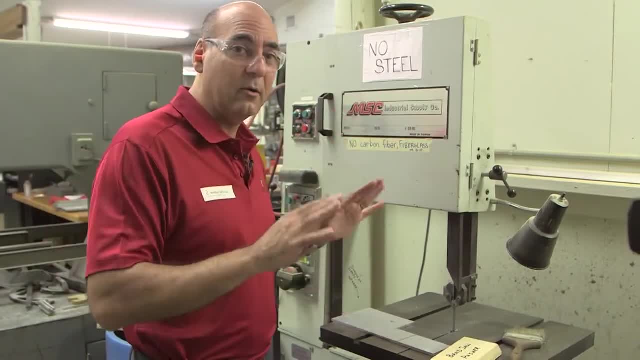 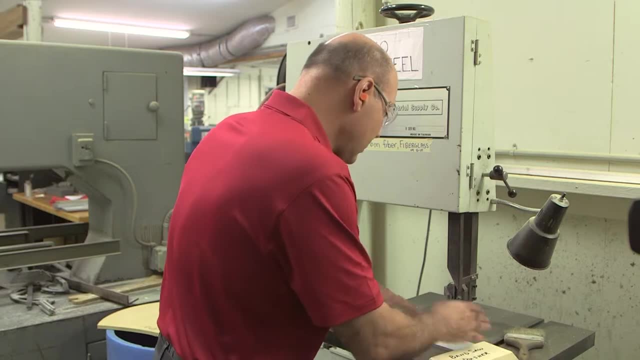 Any other distractions. someone walks in, starts talking to you. you don't pay attention. We're focused here. Say: give me a minute, Wait until I'm done. We're focused on here. Okay, The safety guide. we lower it. 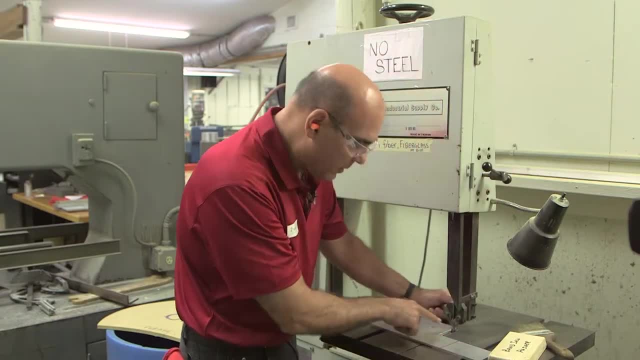 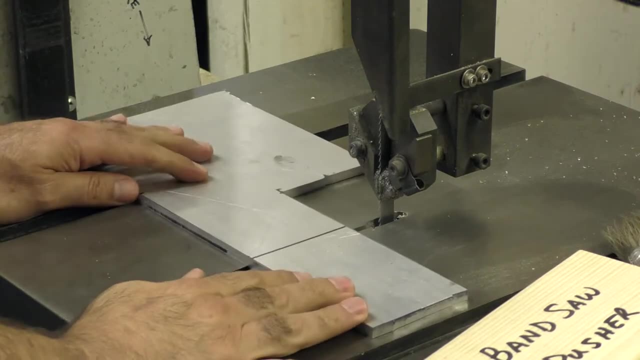 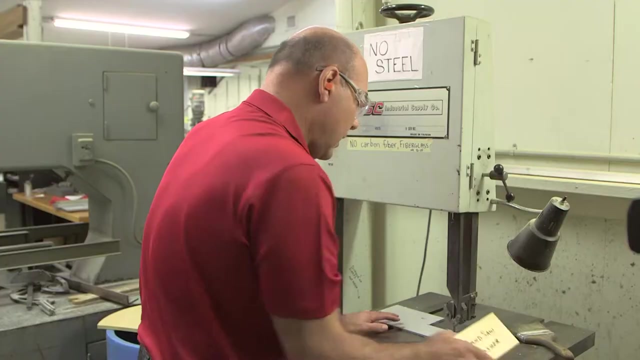 We have to unlock it. We lower it just to above the part. We want to minimize the amount of blade that's exposed. Lift that, Okay, Just relock it. I'm going to cut along this line. I have everything set. 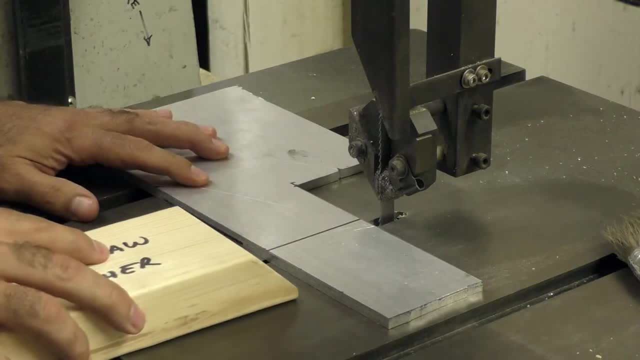 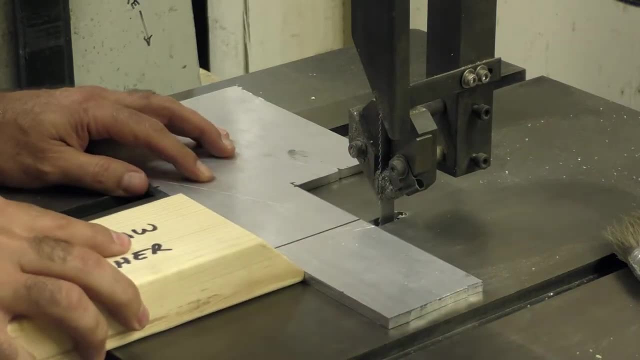 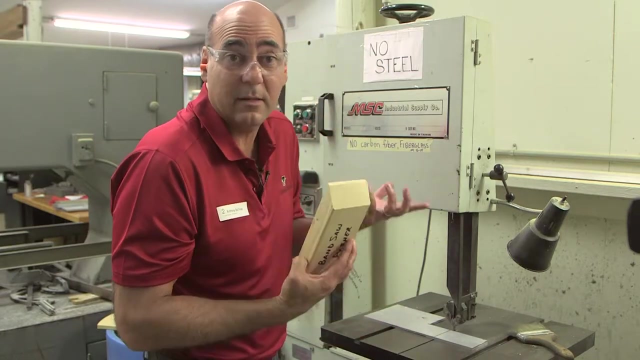 I have a bandsaw pusher. This allows me, when I start to get close to break through, that I don't have my fingers there when I'm breaking through, that I push with this right where the location and where I'm cutting and I push and it's okay if the bandsaw cuts into this. 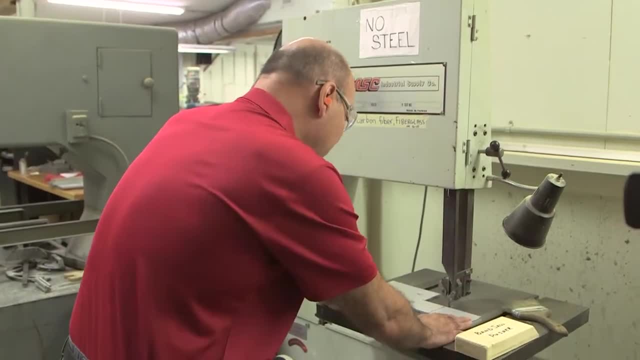 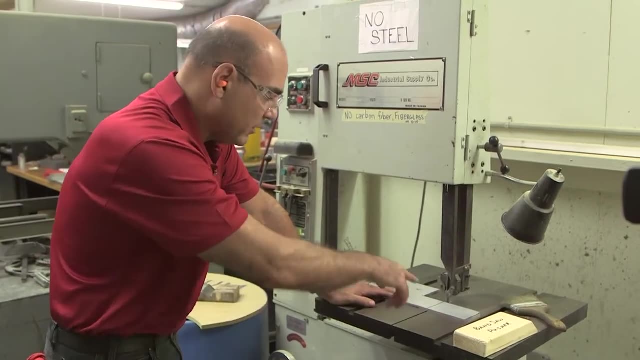 This is just a sacrificial piece of wood. Okay, I have it lined up. The bandsaw will make slight curve cuts, but not so extreme. You can't really force the blade. Okay, Everything's clear, Table's clean, I'm all set to go. 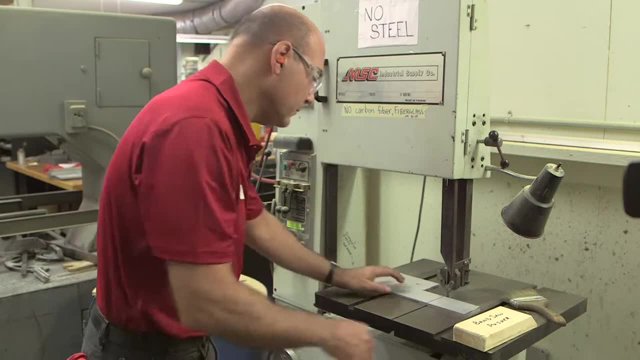 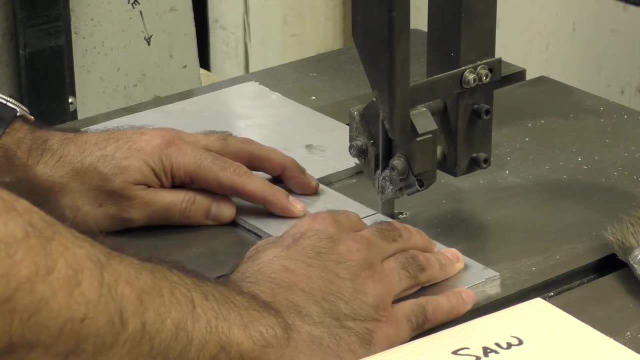 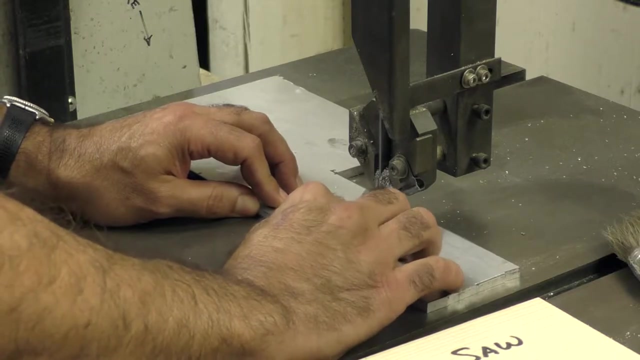 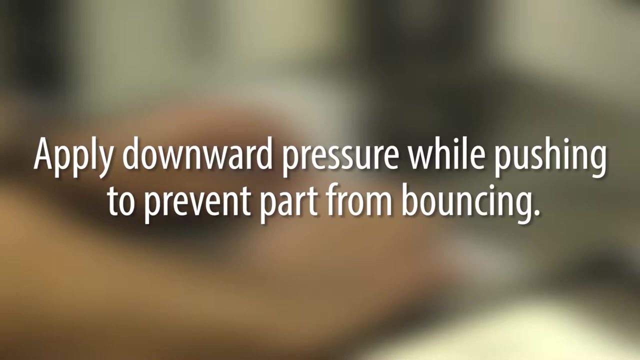 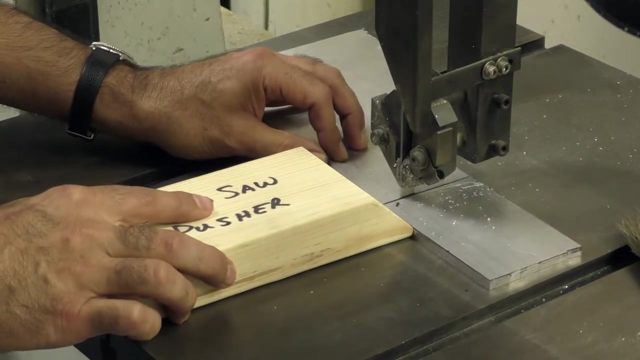 Power on. I want to keep my fingers a couple inches away. I'm going to start cutting. Okay, And I walk my fingers back. Okay, I'm getting close. I'm going to use the bandsaw pusher and I'm pushing right here. 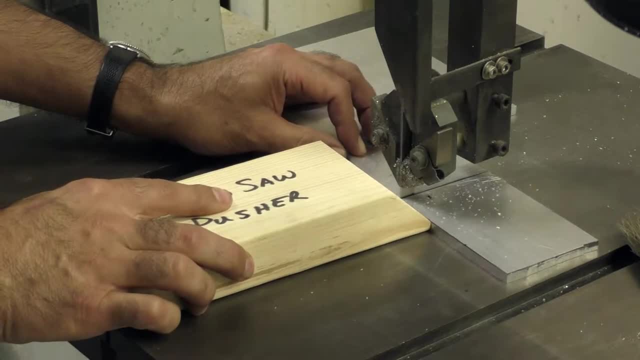 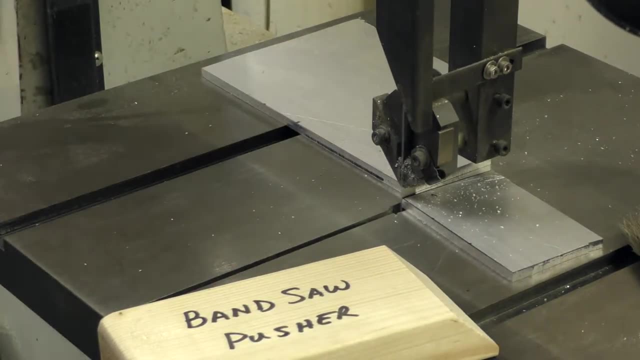 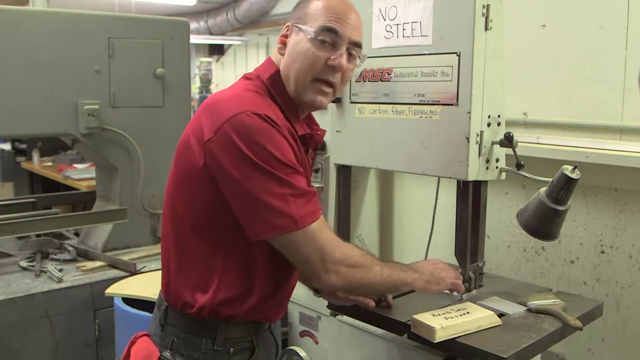 Slow and steady. I'm about to break through, Cut into the thing. I wait till the saw stops. Okay, Before I move any pieces away, I am not reaching to grab a piece As the blade is turning- someone bumps into me. 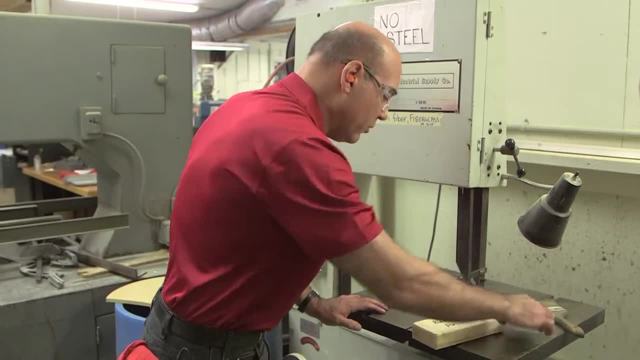 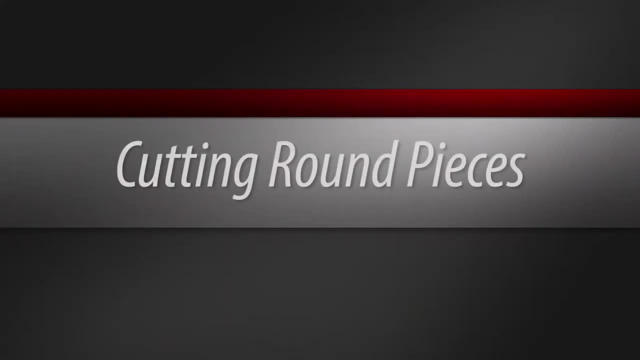 Not a good thing. So I wait till the bandsaw blade stops before I move any pieces away. Any little scrap piece again shut it off. wait till it stops Cutting a round piece. there's no way for us to grip it. 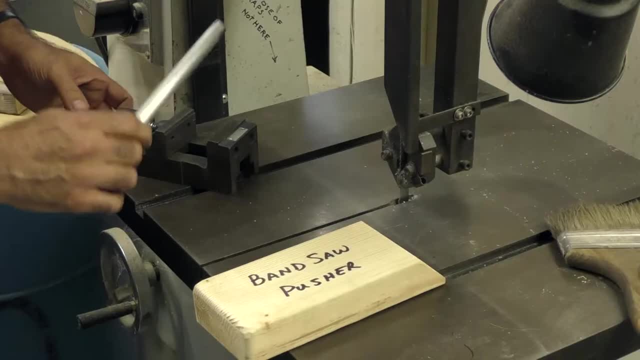 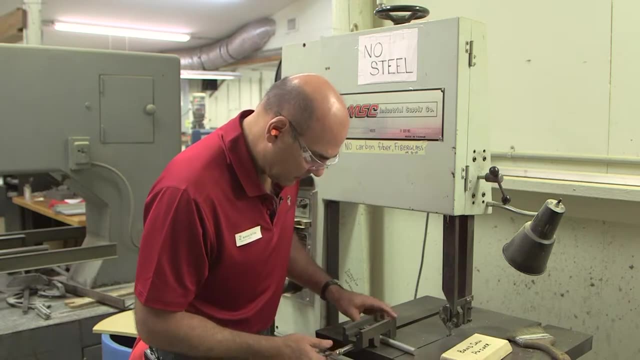 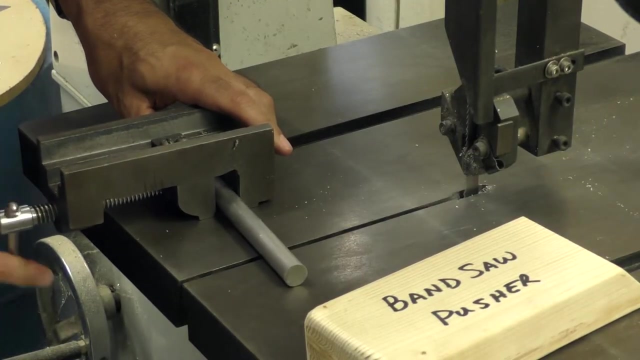 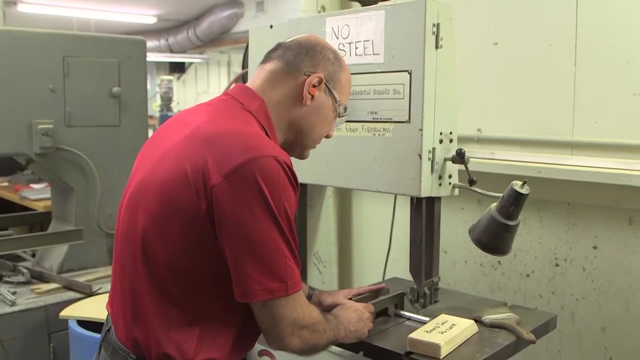 It's going to rotate, We need to use a vice. The way to use the vice on a round piece: turn it upside down So it's held flat up against the table, And then tighten it. Okay, Now, this is a small piece. 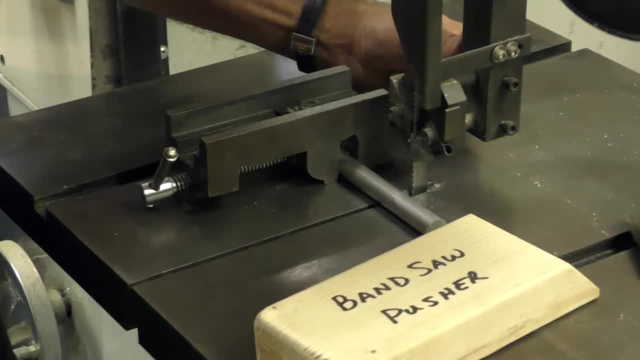 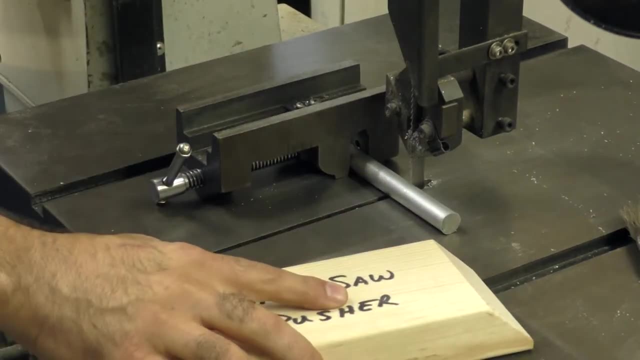 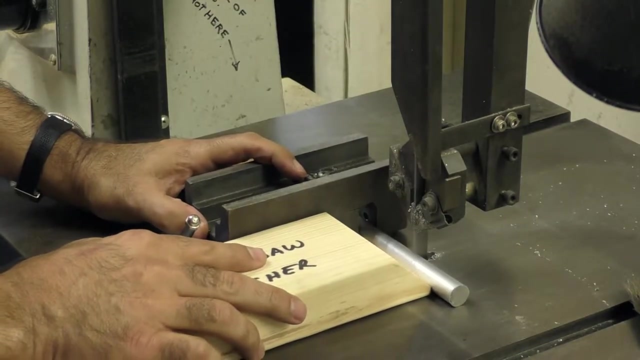 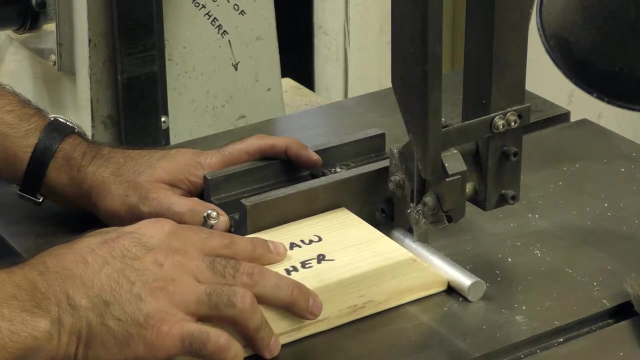 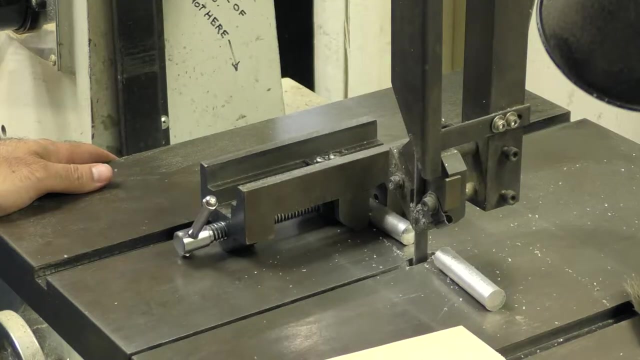 I have to raise my guide, Retighten it, Okay, And I'm going to use the bandsaw pusher Again, focused here. Everything's all set. Press the button on, Shut it off. Wait till the blade stops. 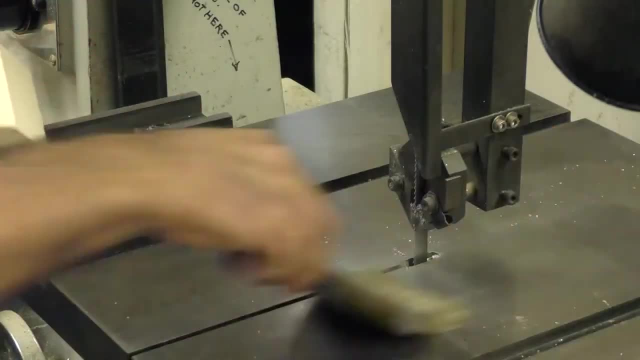 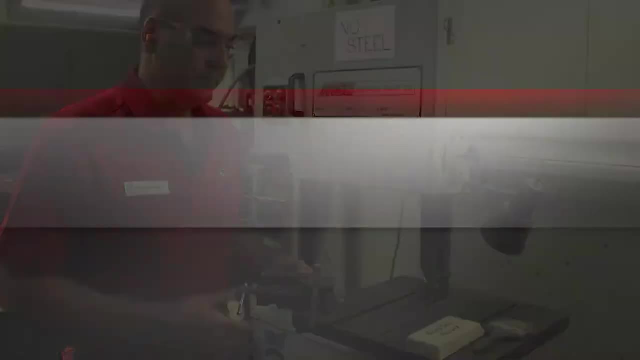 I'm done, Clean it off And I'm going to take a small piece And then I'm going to cut it off and put it in the back of my saw. On to the next. Okay, Here we are on the miter saw. 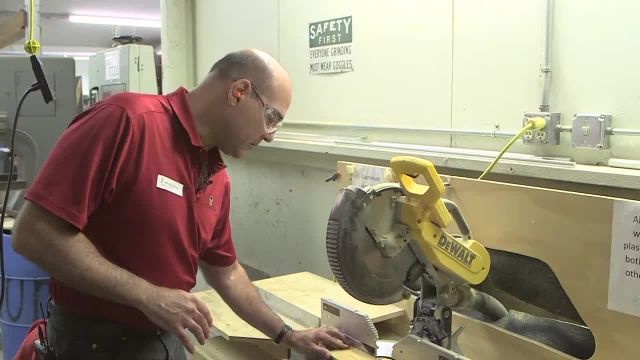 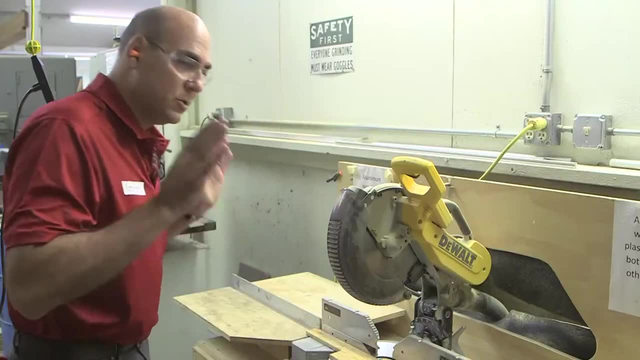 First of all, the piece that you're working with has to be big enough for you to be able to hold firmly. It can't be a small, tiny piece. Your hand's going to be too close to the blade, Totally focused right on here. 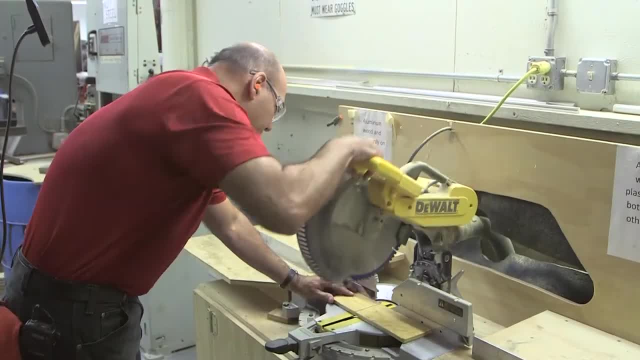 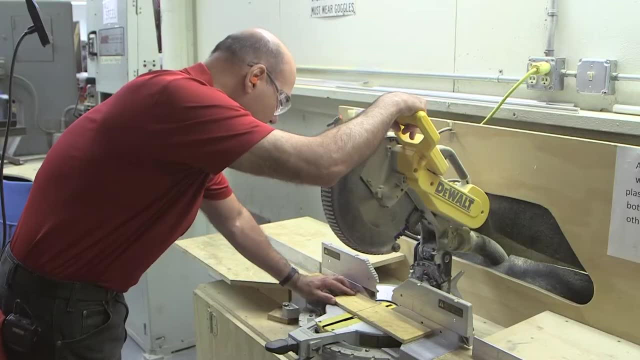 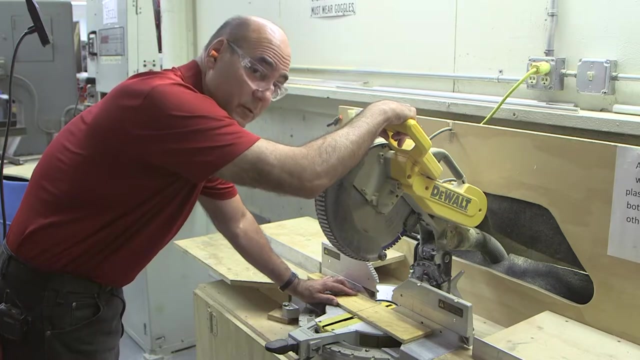 We put the saw up against the fence, Line up our cut lines, line to the blade, make sure we look. okay, we have a good, firm grip. we're holding down up against the face and up against the fence in the back. totally focus. it's going to be loud. here we go, we're going to cut through the piece, release the. 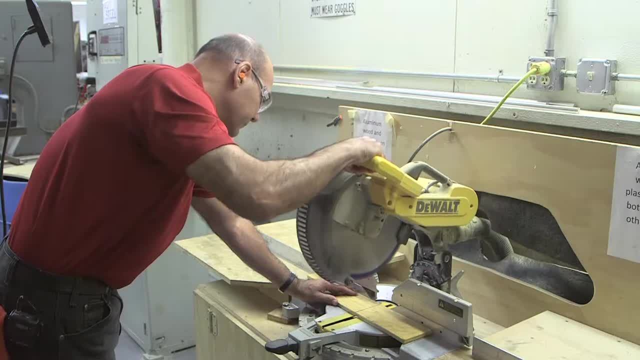 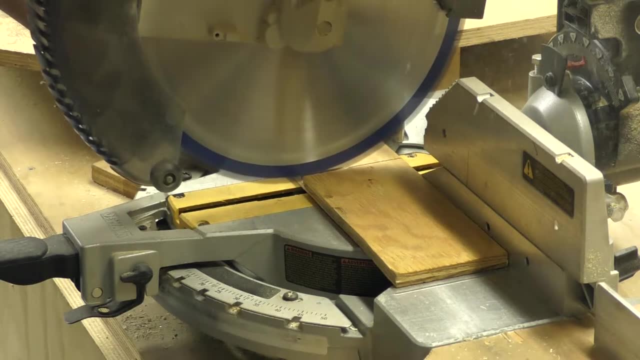 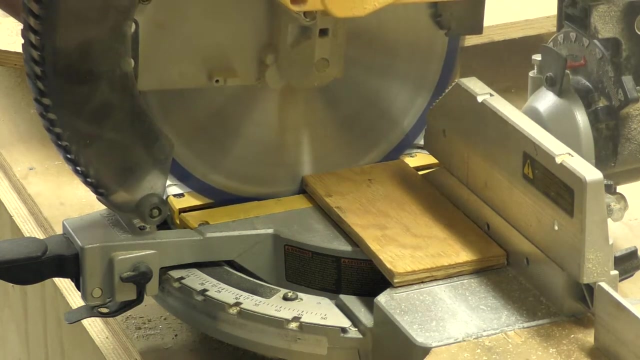 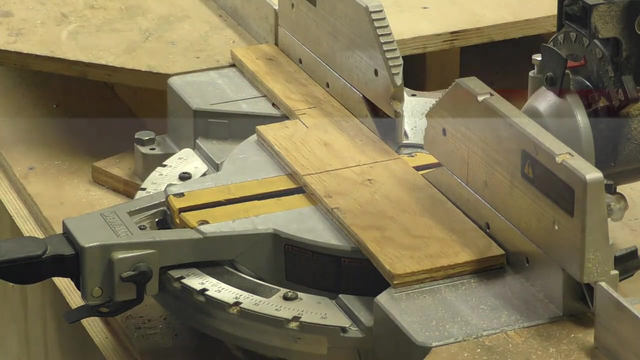 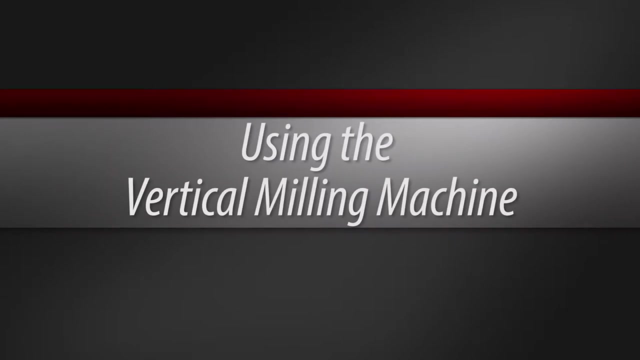 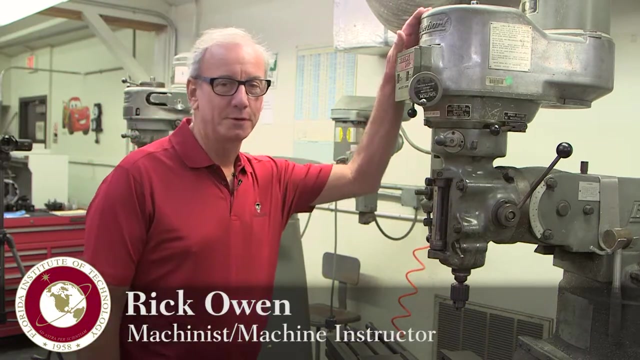 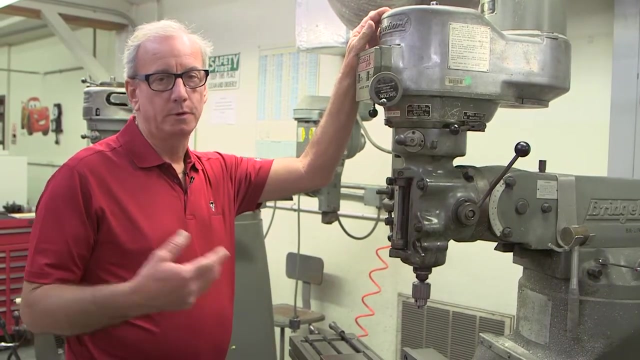 trigger, wait till the blade stops, then bring it up. that's it with that. welcome students to our Florida Tech YouTube video presentation. this is our vertical milling machine. what I'm going to do is refresh how we approached the machine when we're starting to work, because there's been some problems in terms of how to put the 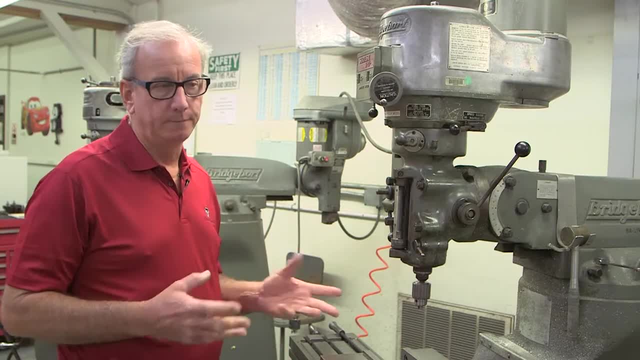 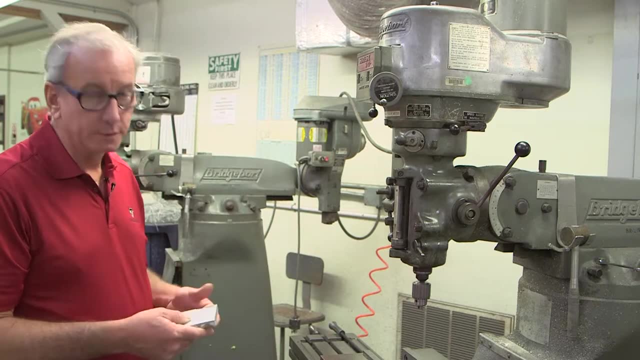 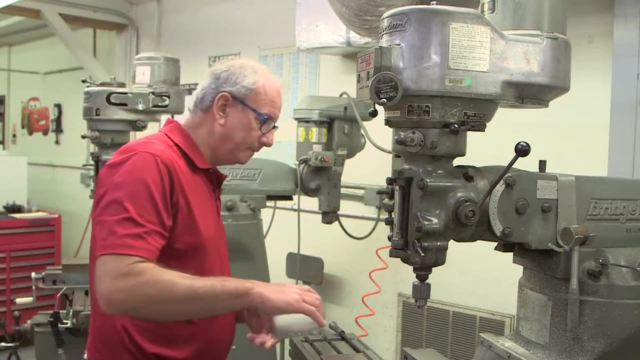 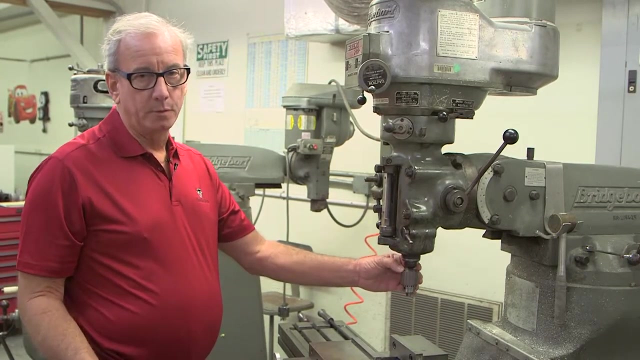 tools and take the tools out and various other elements. so we have a part. we need to mill it square. so the first thing we want to do is set the machine up to mill this surface here. so we see we have a drill chuck in here. this brings up an important point: is we do? 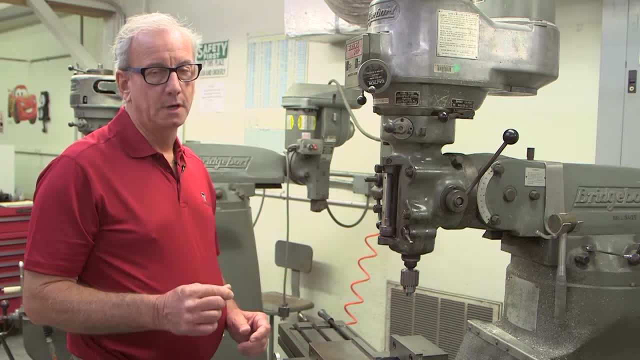 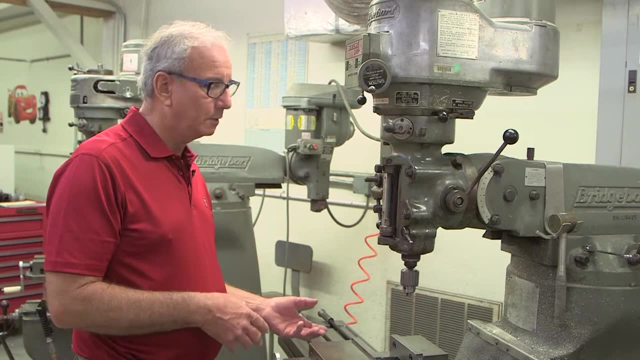 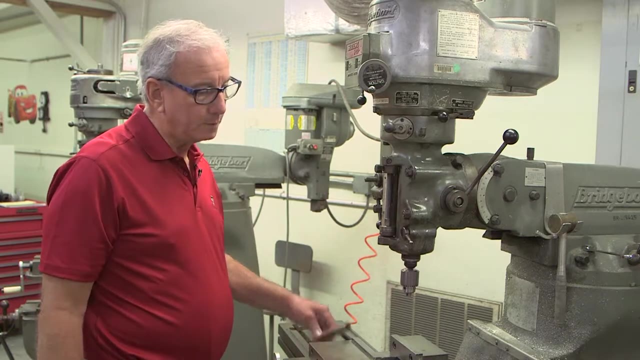 not put drill bits into collets. we only put drill bits into the drill chucks. so if you're going to use the milling machine to drill holes, we need to put a drill chuck into the machine. but right now we want to do, we want to put a. 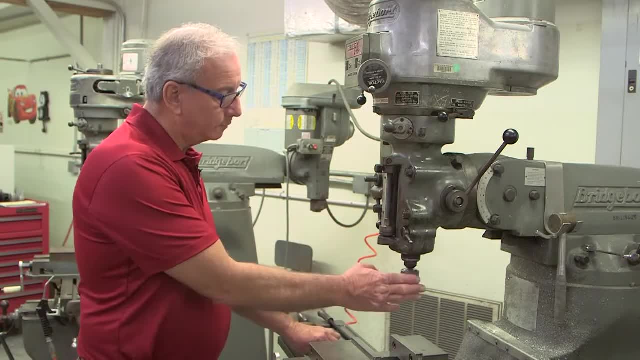 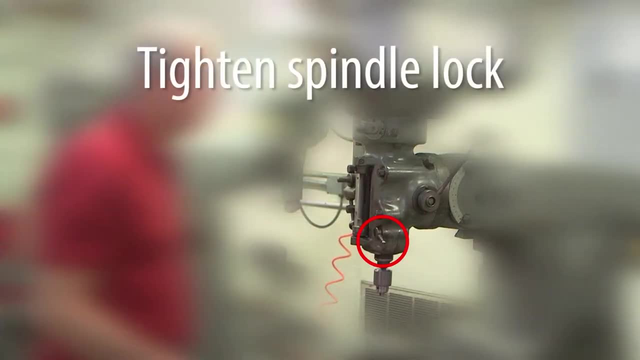 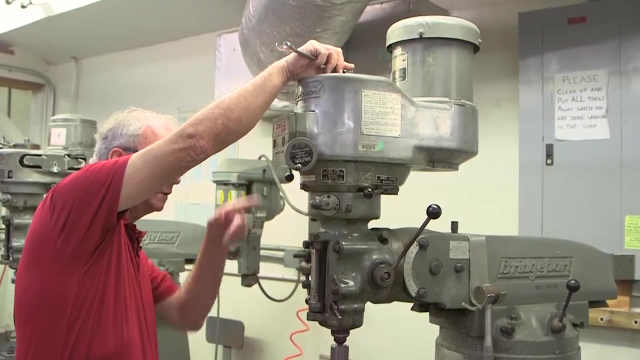 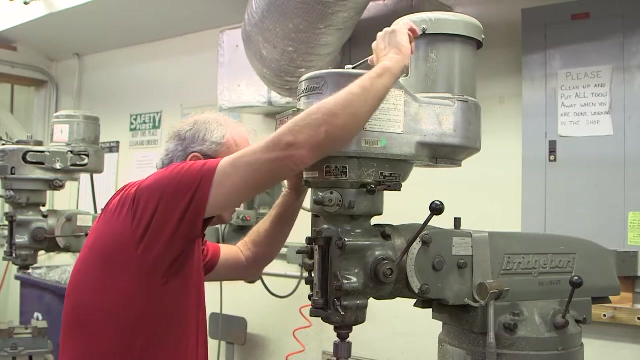 milling cutter into the machine. so we need to take our drill chuck out. so we take our 3 quarter inch wrench. we put it up on top of the draw bar because we have to unscrew our draw bar to release the drill chuck. we put on the brake, release the draw bar about a half. 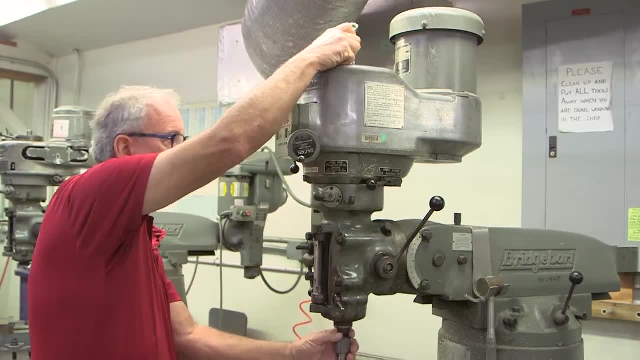 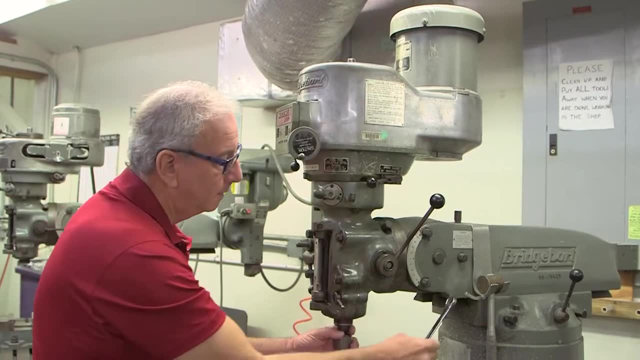 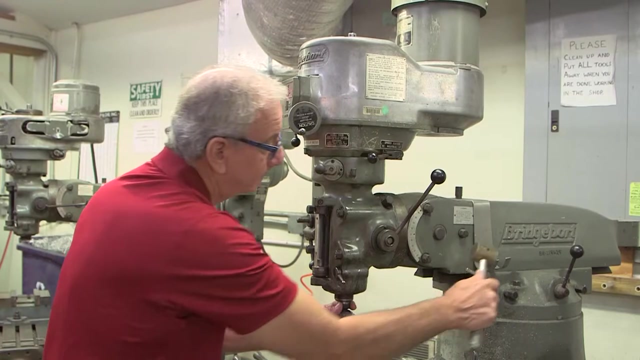 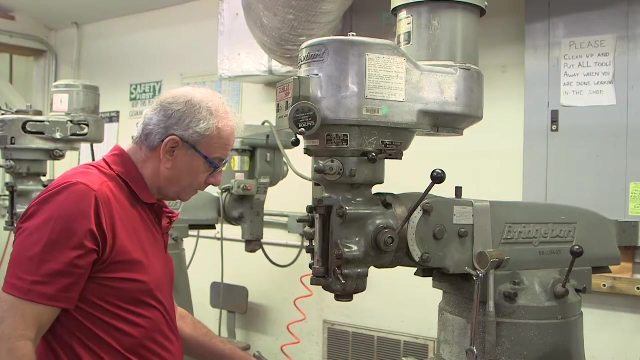 a turn, half a turn only. then often you can just take and tap the draw bar with a wrench and it'll come out. other times it won't come out and you have to use a nice brass hammer- this time it came out quite easily- unscrew the draw bar and take the drill, chuck out. so let me show you what. 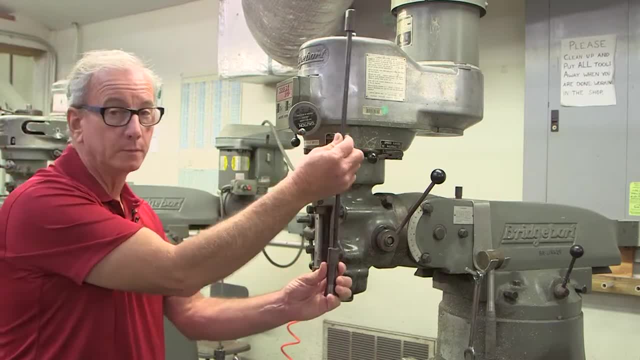 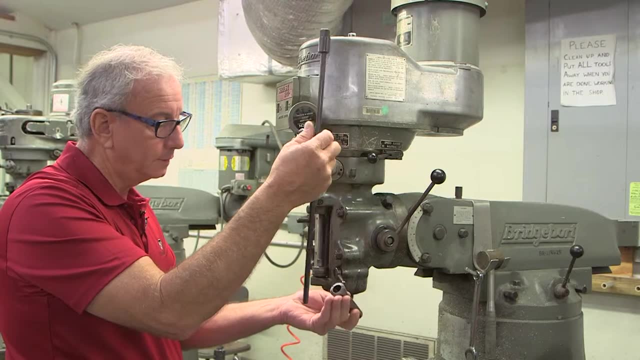 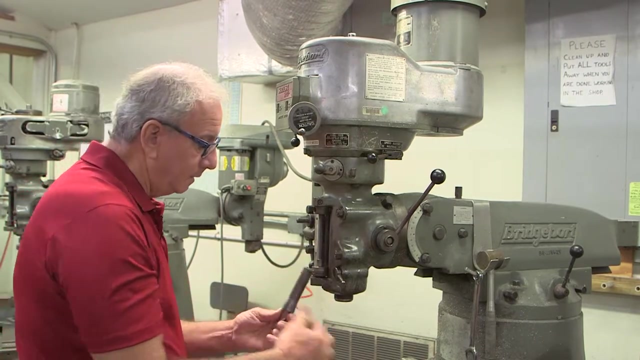 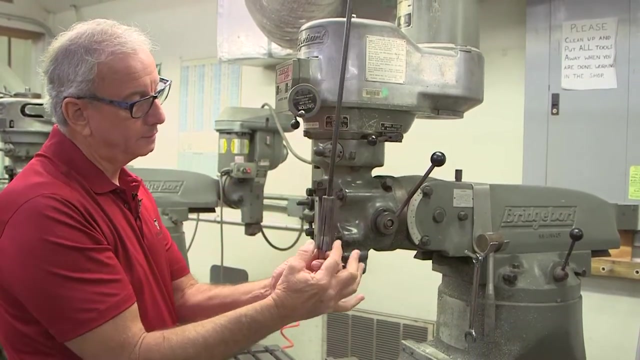 the draw bar is. this is actually the draw bar that runs down through the, the spindle and this is actually a collet. So what we're doing is we're putting our cutter- whatever type of cutter or drill chuck- into the collet, inserting the drawbar, and then, when this tightens, it pulls up against the taper. 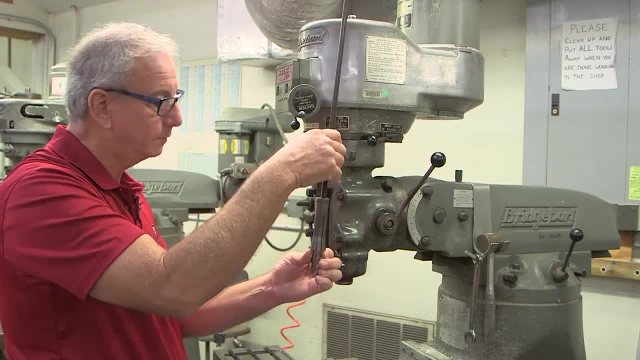 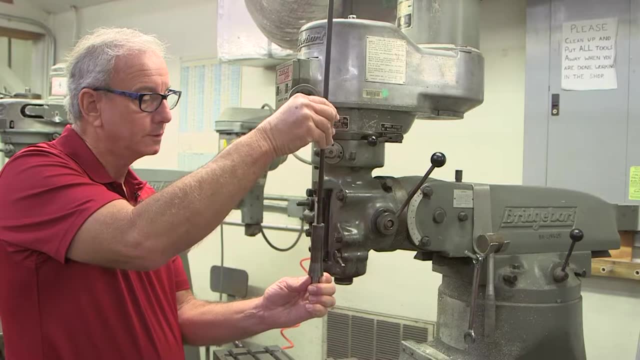 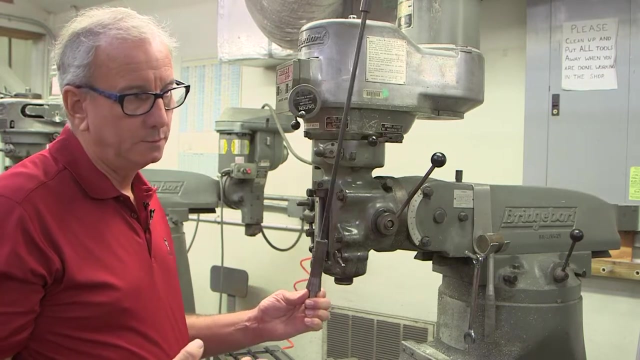 here which locks the cutter or the drill chuck into the machine. So when we go to take it out we unscrew the drawbar just a little bit and then tap it. What one thing that's been happening- and we lost three drawbars last year in one week- is 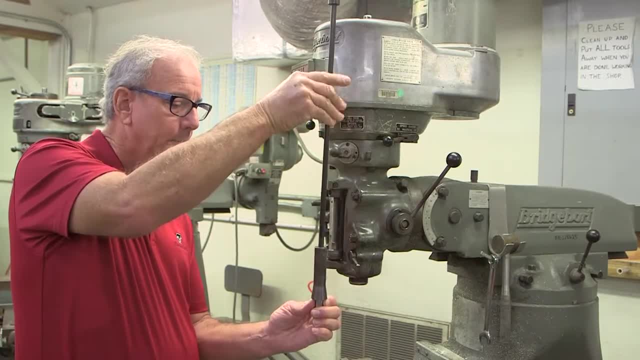 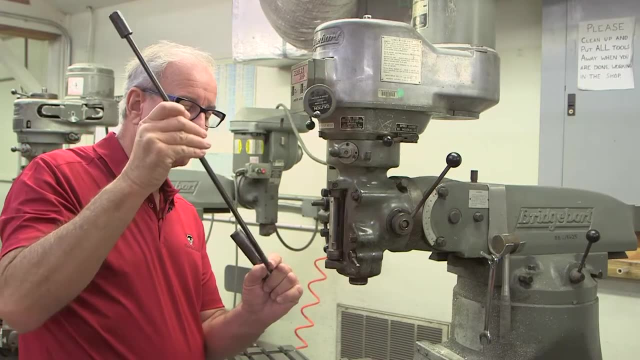 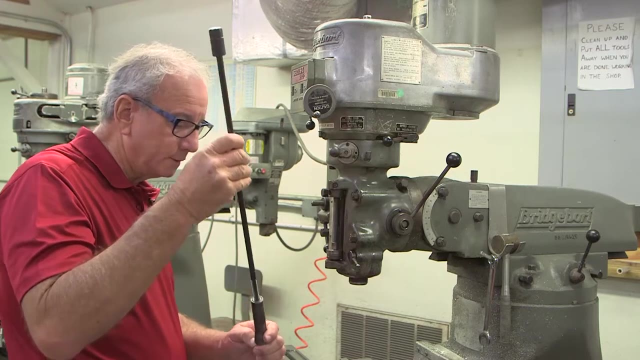 the students will unscrew the drawbar and completely from the collet, then take the brass hammer and pound it. What happens if that happens is it rolls the first threads of the drawbar and pretty much ruins it. So the crew correct way is to unscrew only a half a turn If you have to whack it with a. 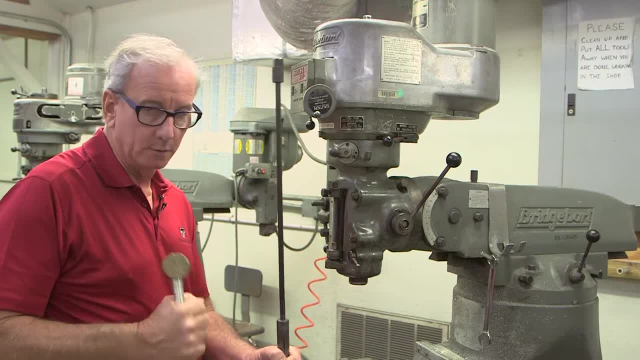 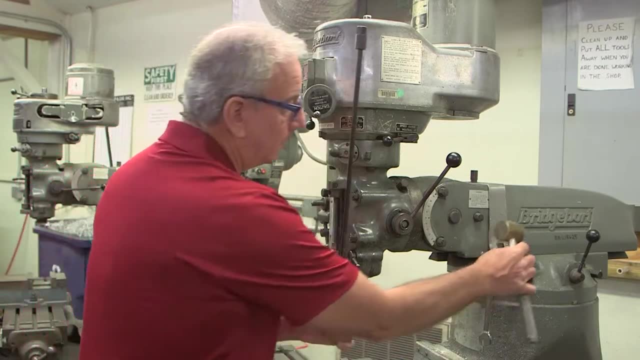 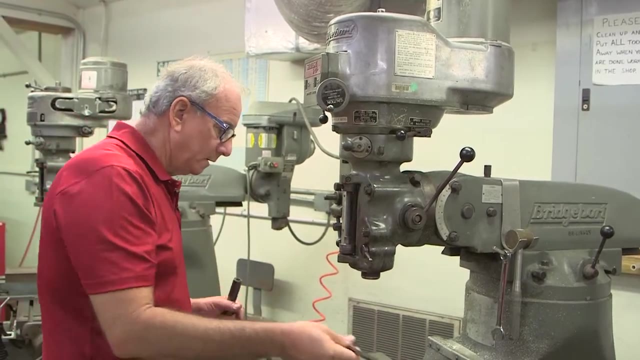 brass hammer. you can give it a really good pop, or two or three or whatever it takes to release the taper onto the collet, and you do not injure the drawbar because there's enough threads engaged that it won't get mutilated. So now we 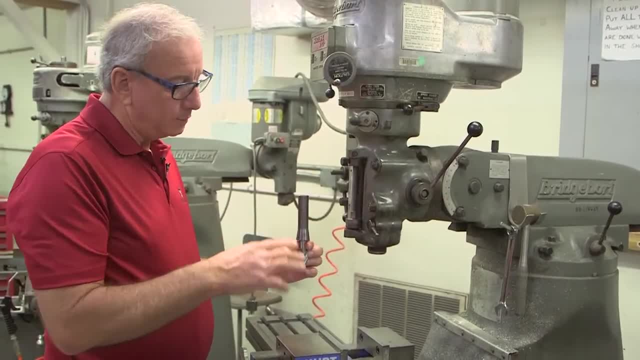 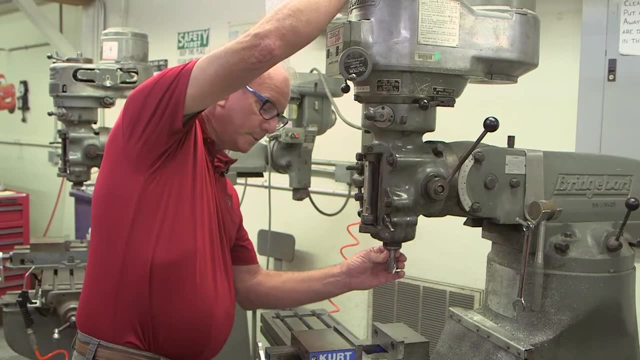 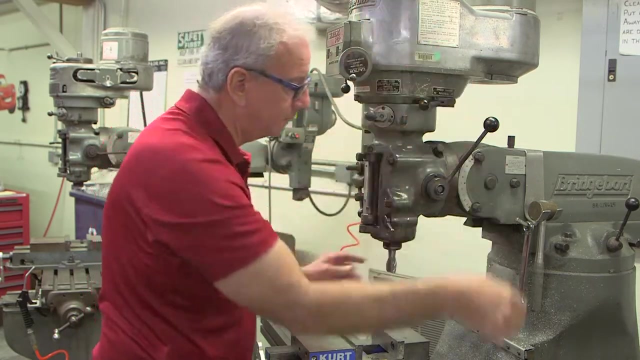 want to put our end mill into the machine, because we're going to mill the corner of the, the plate We insert like this: reach up here to the drawbar and screw it down into the collet. At this point we take then our wrench again, put our hand on the. 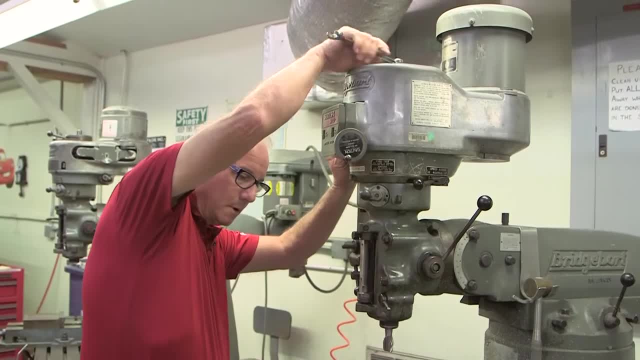 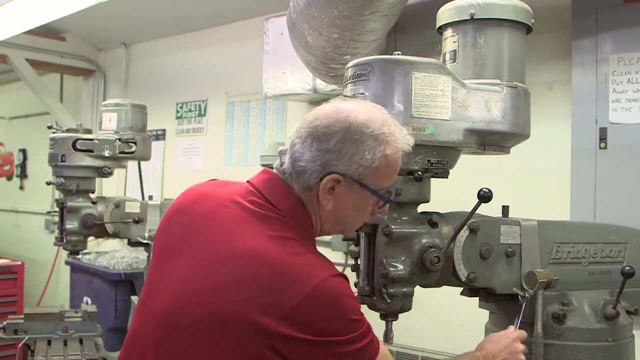 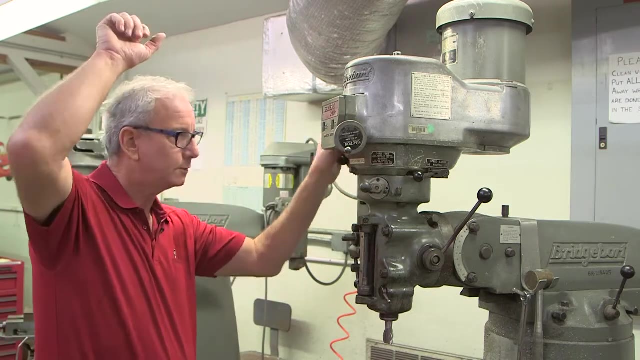 brake wrench at the top of the drawbar and we tighten it and all we have to do is just firm it up. Twice students have tightened it so tight that I had to go get a pipe and put it on top of here and push while he held the brake to unscrew it. 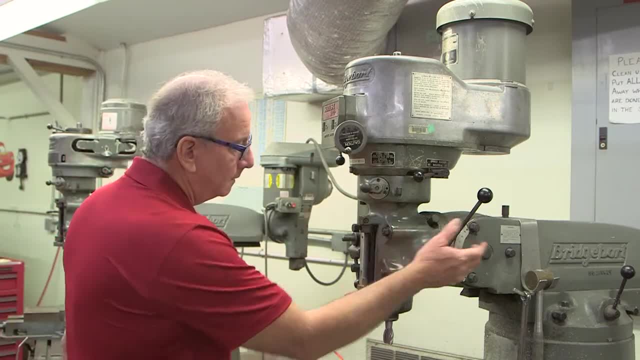 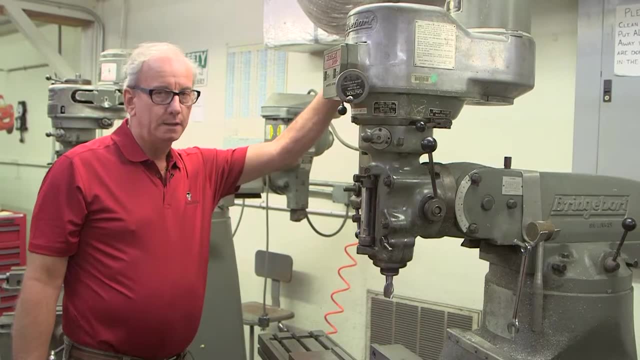 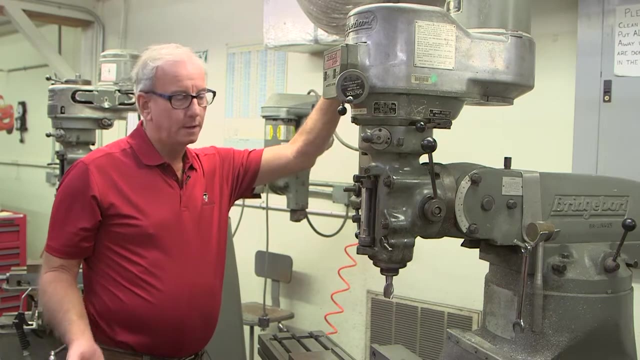 It doesn't need to be that tight. The next thing we do we need to know how to turn the machine on. This switch has a high and a low. Depending upon which you go to high or low is depending upon the rotation of the cutter, So I'm gonna switch it one way. 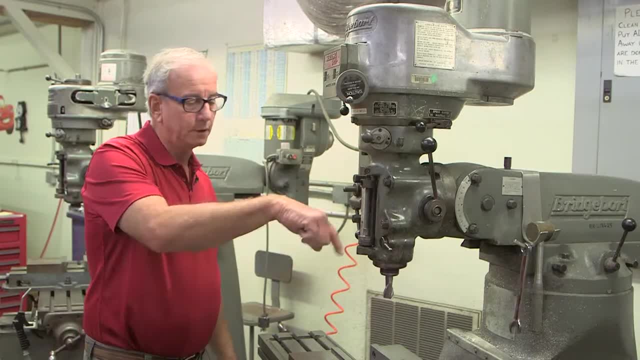 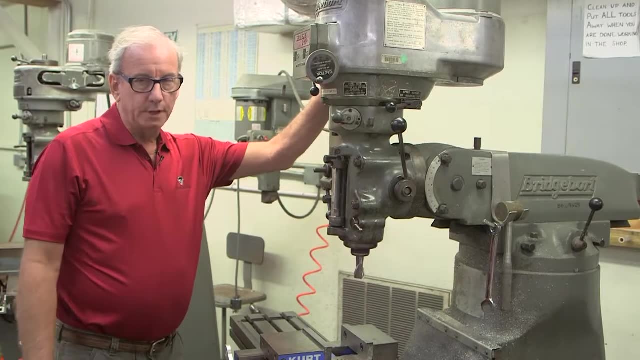 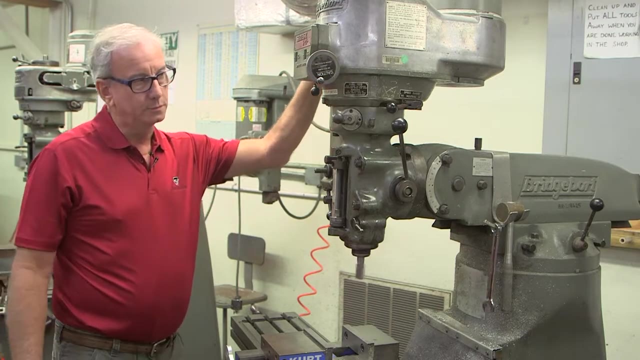 Notice that the cutter goes in the correct direction, which is a clockwise direction. as you're looking down, The switch has two, two positions, like I mentioned. If I turn into a low, it's going to turn backwards. This is part of our machine shop. 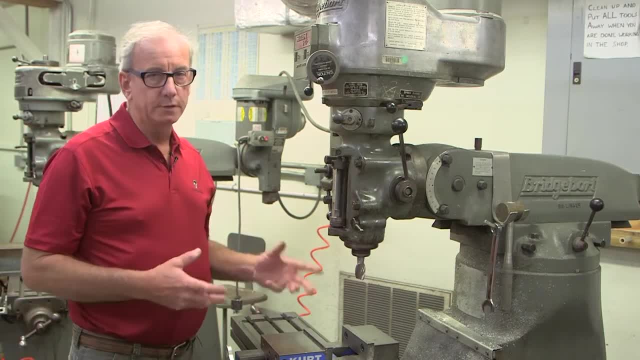 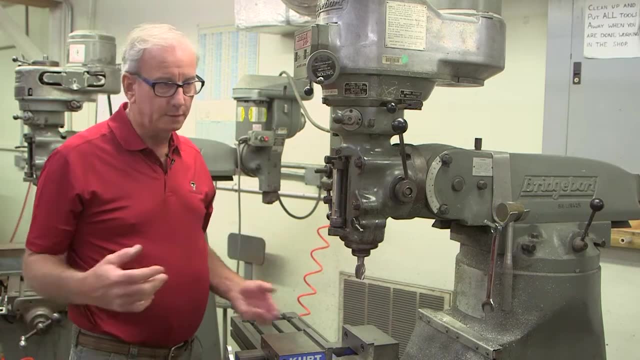 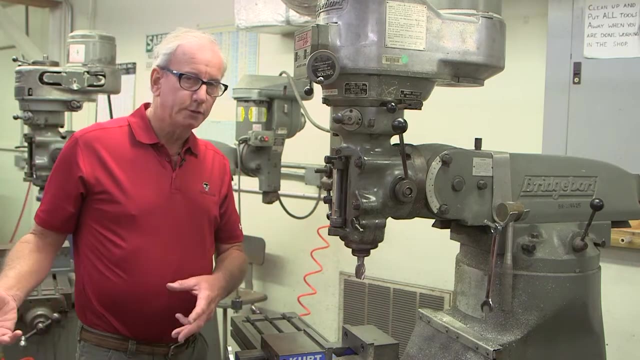 training, and it's called awareness. This is a real Zen type environment, Zen being that if your thoughts are going a hundred miles an hour and you're thinking about this and that and the other, then those block your attention. We have to shift our our attention from thoughts to work, to being. 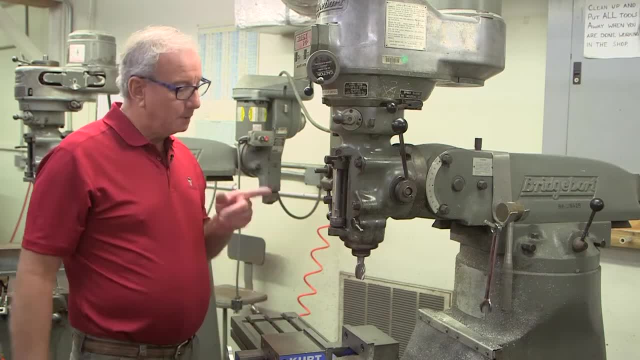 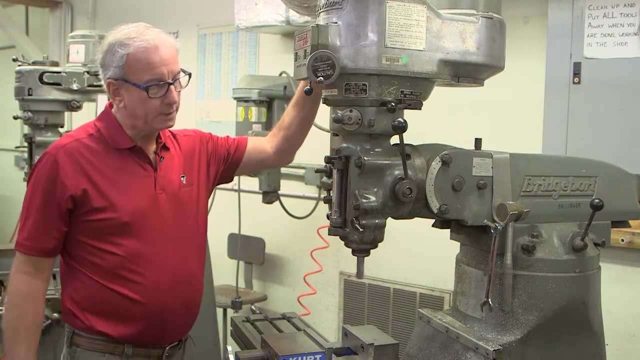 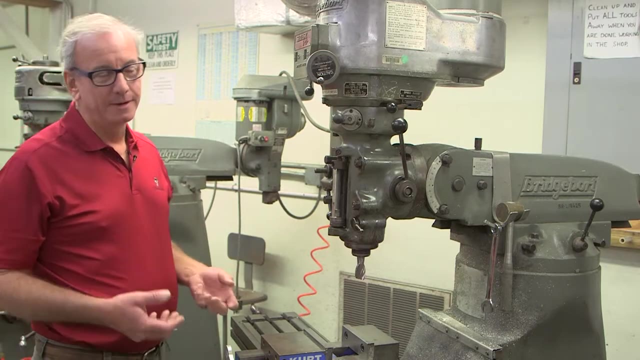 here present now Zen. So first thing you do when you turn on a machine is you watch which way it cuts. If it's turning counterclockwise, we got a problem. The problem is it won't cut. It destroys the part, destroys the cutter. So that's thirty thirty dollars down the drain and this happens. 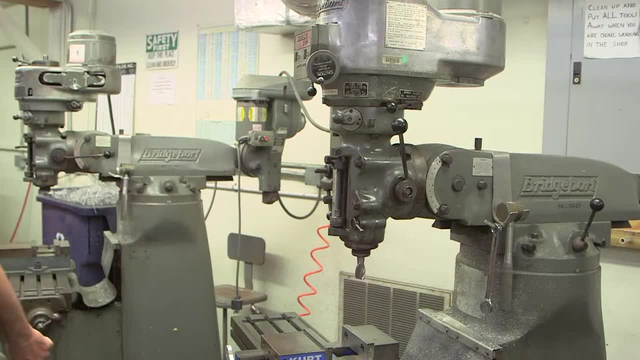 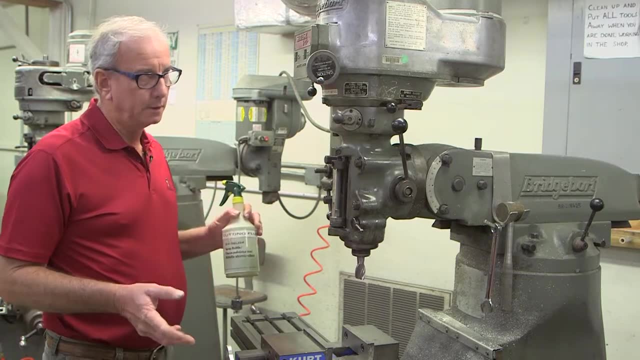 quite often. The other thing is, when we do use our cutter, we use our cutting fluid It's. it's very much like it's a soluble oil, very much like dish soap That can be used as a cutting fluid. It's a soluble oil, very much like dish soap That can be used as a 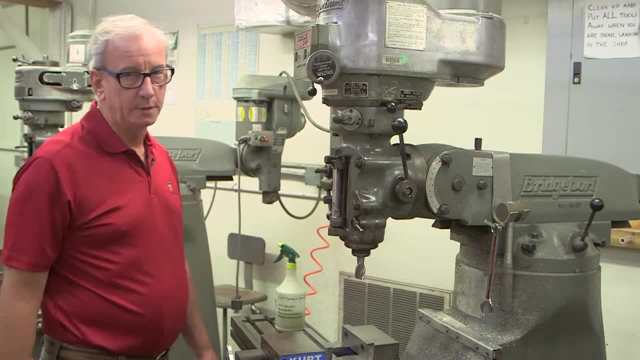 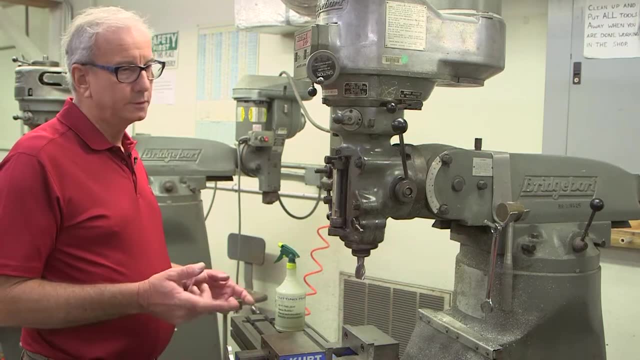 cutting fluid. It's a soluble oil, very much like dish soap, That can be used as a cutting fluid That keeps the aluminum or steel from gumming up and ruining the tool. Okay, one of the things that happens when a student turns it on backwards is he says: well, this is a stupid machine. It's got two. 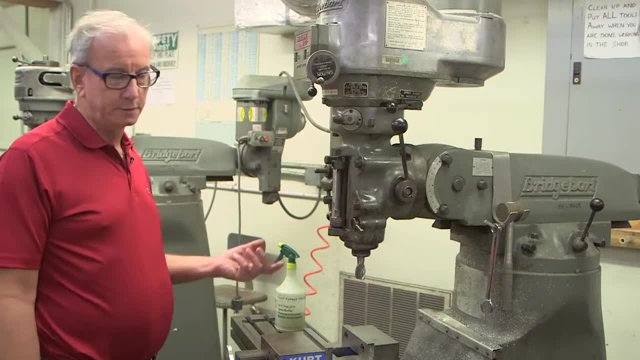 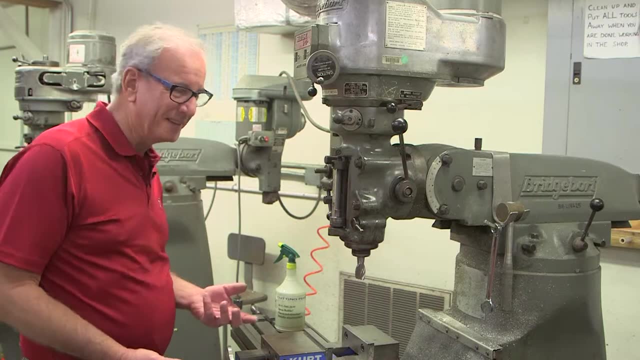 positions. It's got a high and a low. Why doesn't it turn on? just like my fan, It only goes on in the right directions. Well, there's a reason for that and it's not a stupid machine. It has a what's. 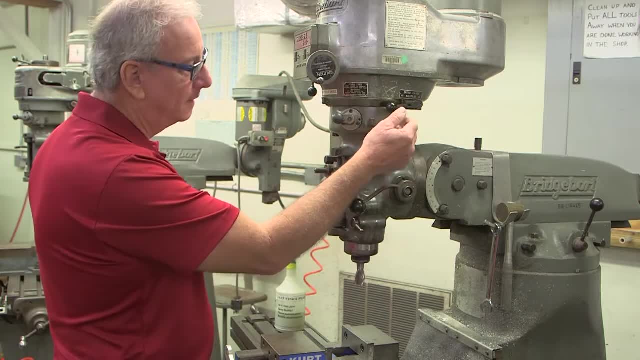 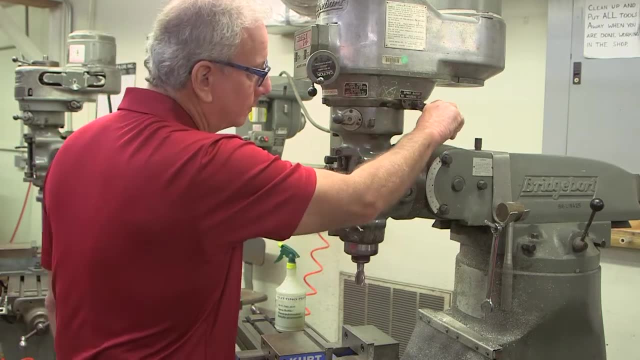 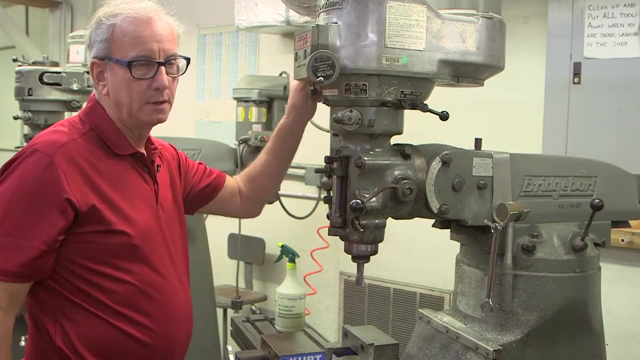 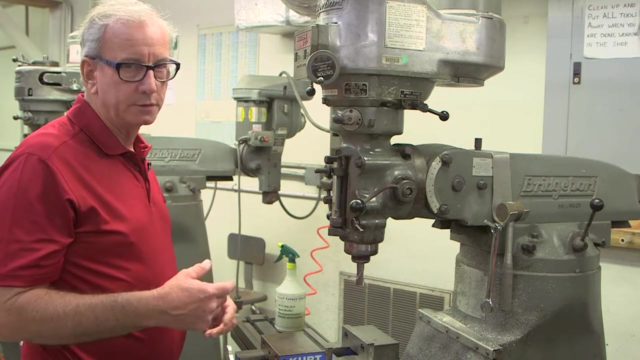 called a back gear. This is the back gear. What happens is it's in high range. now If you push, push this knob in, move it towards the back, Then you turn the machine on to low. It's going to turn in the correct clockwise position, but much slower. So we have a back gear for turning really slow. 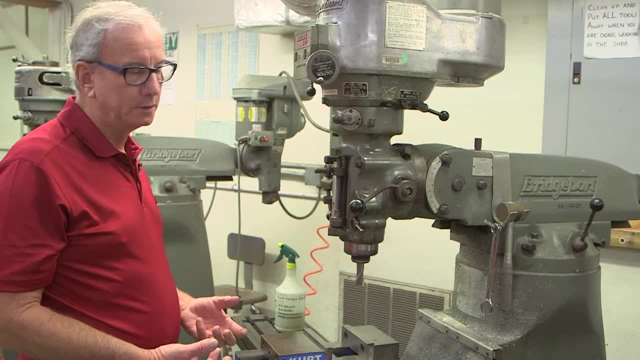 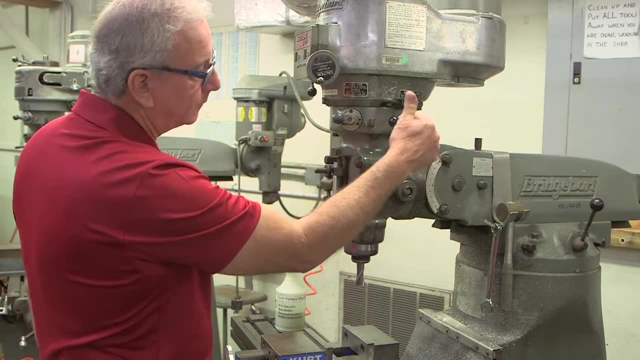 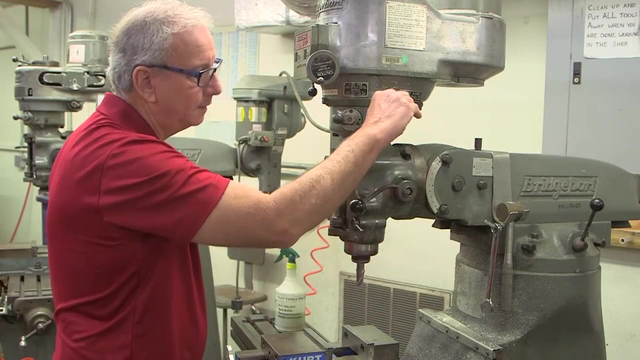 drilling really big holes, cutting really hard material, Then we have a the forward position high. Notice that when I move this over here it didn't go all the way. You must grab the spindle, give it a shake and then it will pop into your high range. If you don't do that- and 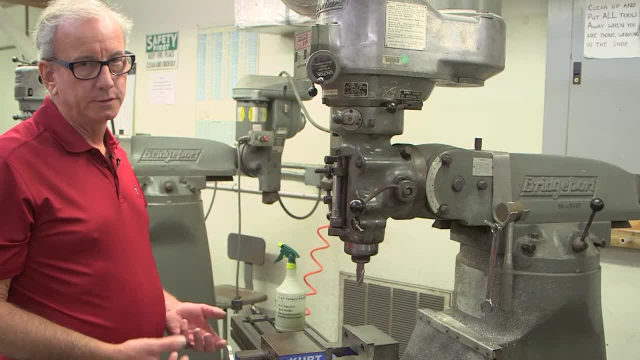 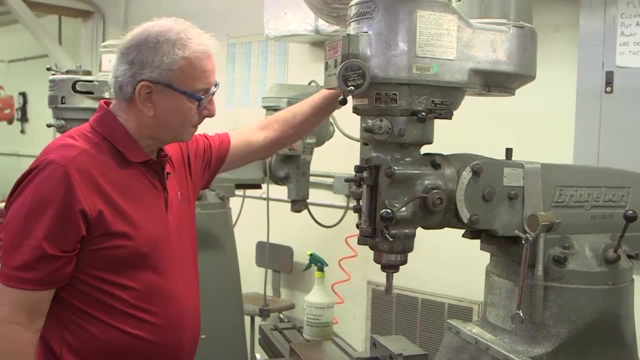 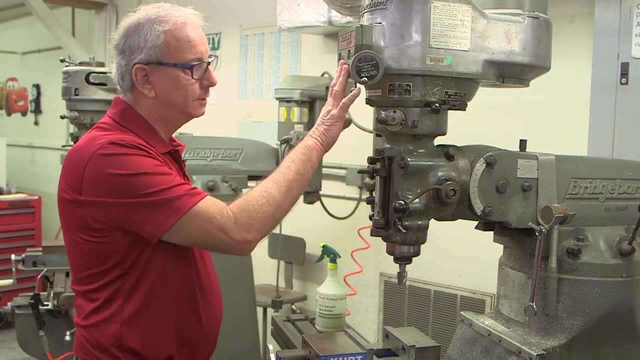 turn the machine on, it'll make the loudest, loudest, ugliest noise you ever heard in your life and be very embarrassing. So, okay, right direction. It's still maybe going too fast. This machine is a variable speed, So we turn it on, We can slow the speed. 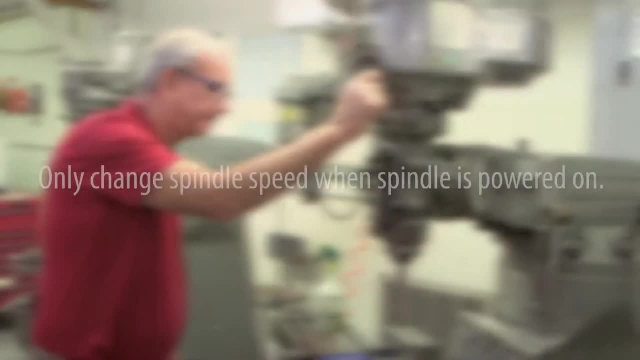 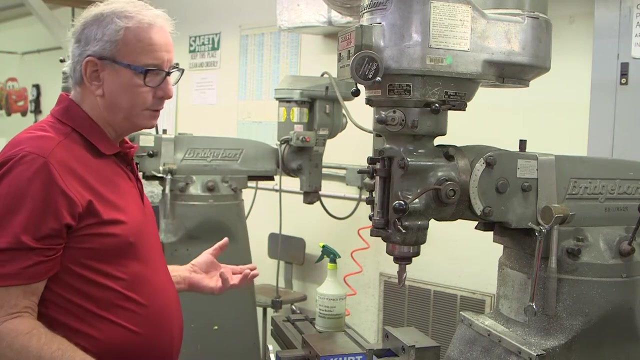 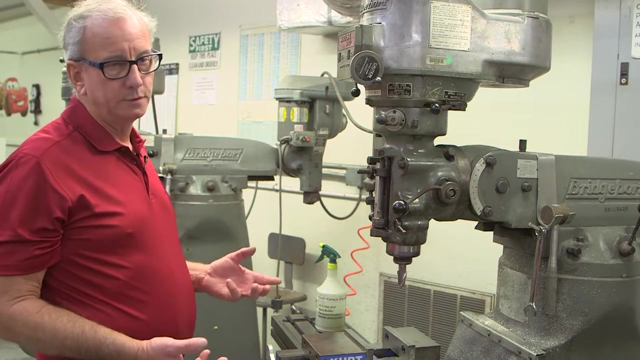 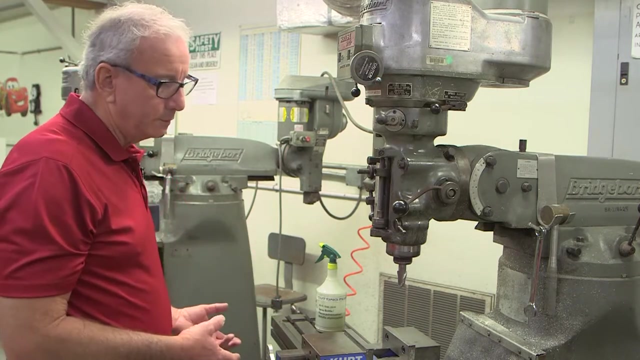 down or speed it up with the variable speed. knob Speed is very important. That comes to another situation As we, as Most students, don't always know the correct speeds and feeds and whatever to use. so that's when you come up to me or Anthony or Bill, and say, gee, I'm not really sure. 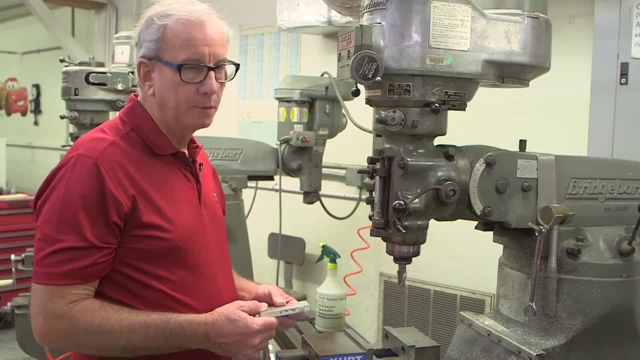 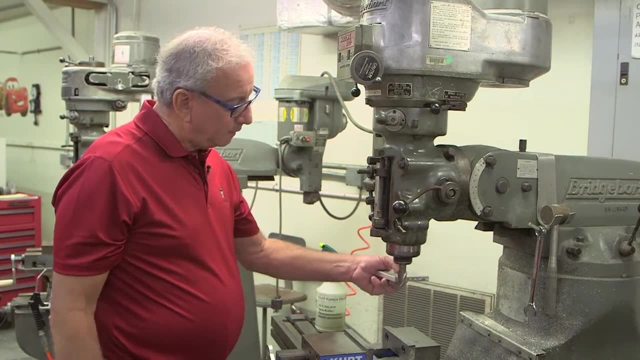 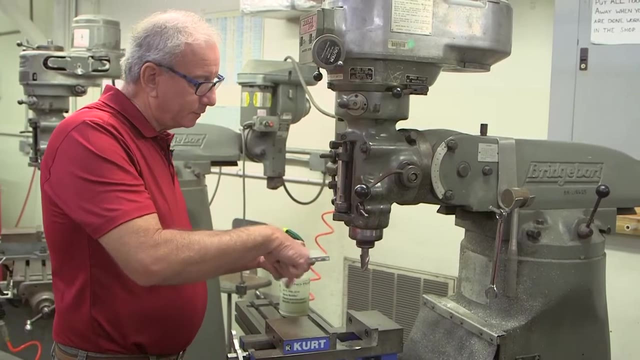 We'll step in, we'll help you out. The last important point that I want to address is the difference in the way you can mill a part. If this cutter is turning clockwise and we come across this edge here, then that is conventional milling. 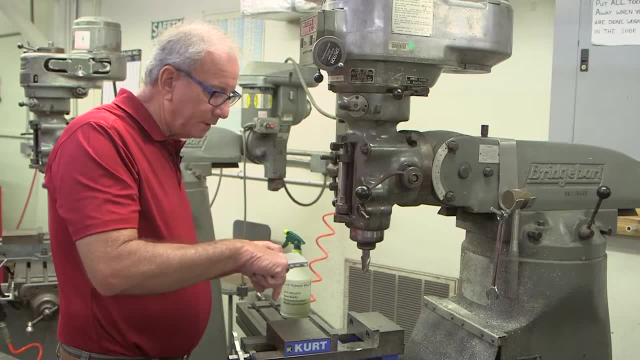 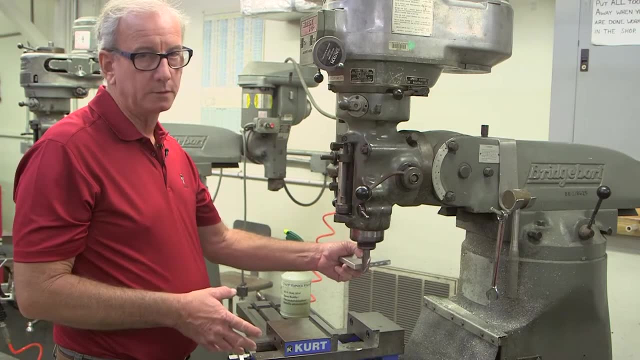 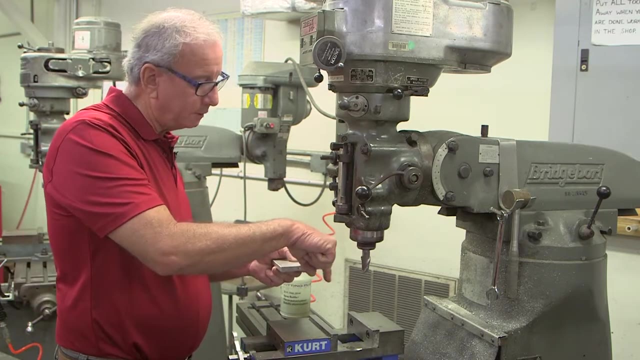 So the part actually progresses into the edge of the cutter. That's the safe way to use these manual milling machines. If we go in the opposite direction, it's called climb milling. That's where the milling cutter is going, also in this direction. 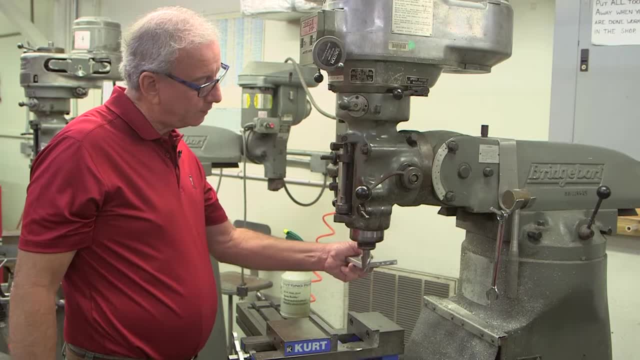 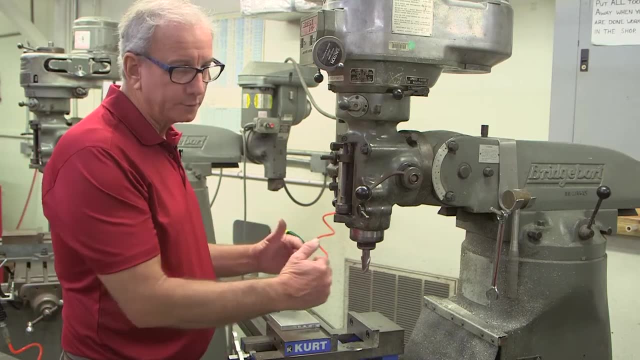 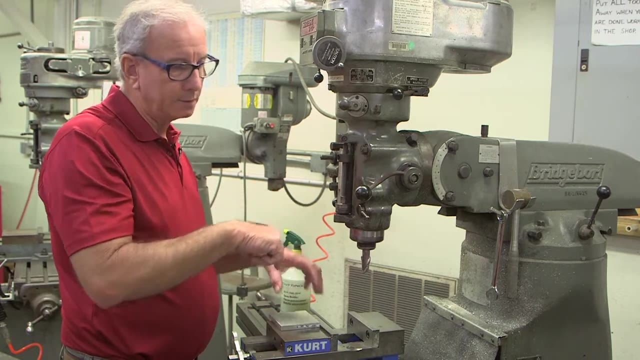 What we're climbing. we're actually climbing on top of the edge. That's not safe on these machines. The reason why it's not safe is that the tables are very, very loose and they can shake. What'll happen is, as it climbs onto the part, it'll grab ahold of the machine and pull it. 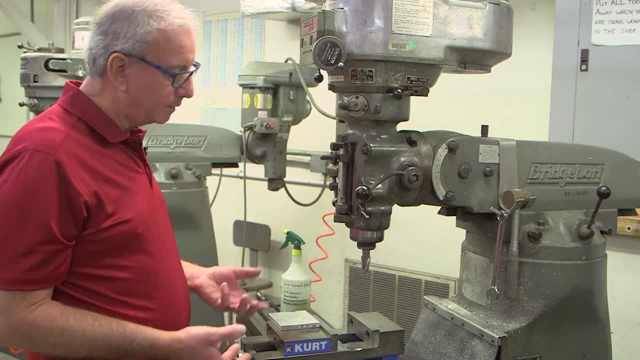 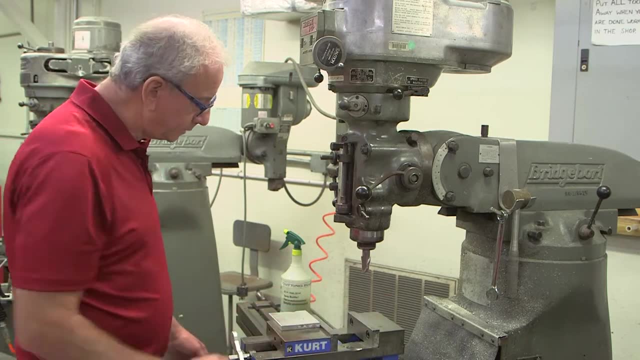 into it. At that point it can break your part, break the cutter and cause some problems. The one last thing I want to mention is, If you're milling in this direction, there is a lock, a table lock, on this side that. 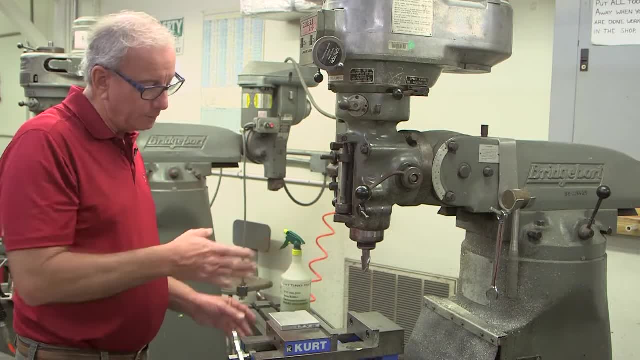 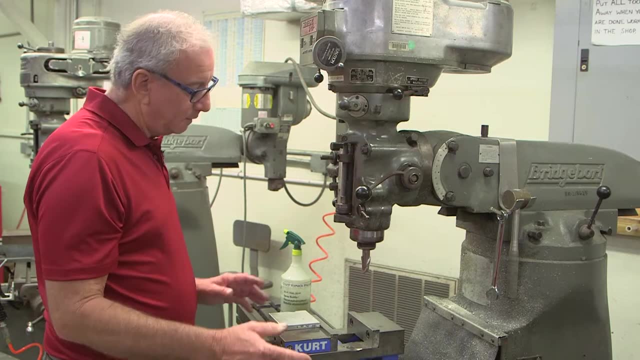 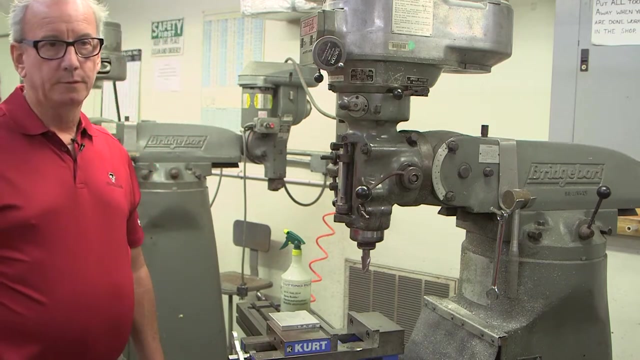 you can put on to keep the table from drifting as you're milling across it. If you're milling in this direction, you can use a table lock here for the X. that'll prevent the table from moving this way. That's about it for the vertical milling machine. 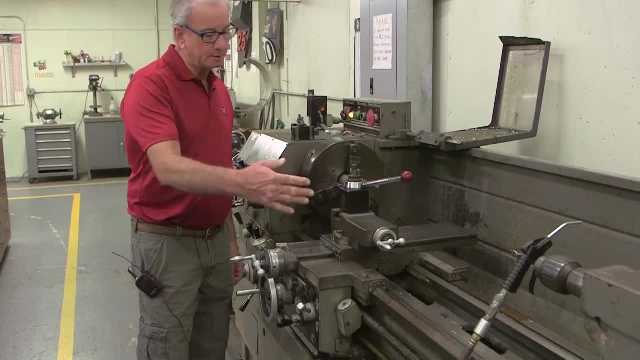 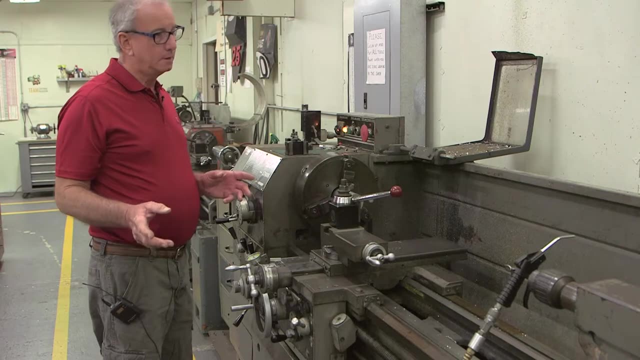 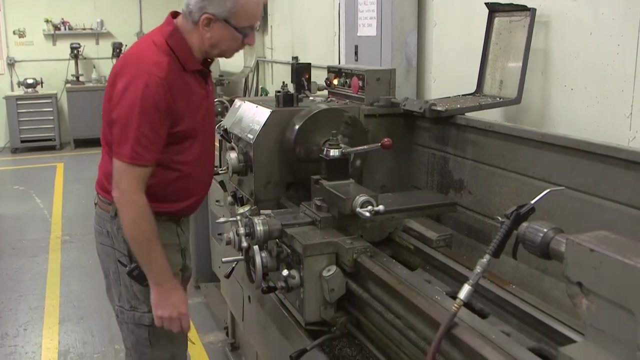 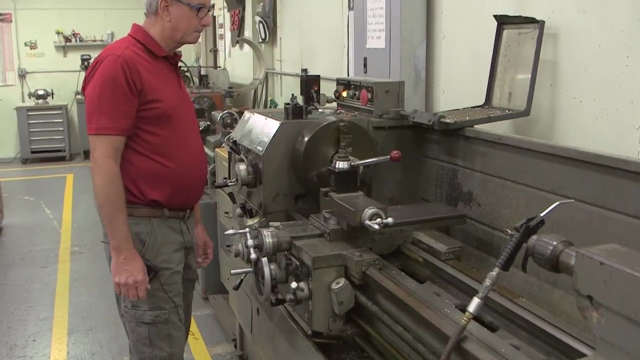 This is the engine lathe. This handle moves it back and forth this way. This handle moves it this way. One of the problems we have in the past is turning the machine on. This handle turns it on and it rotates in this direction. 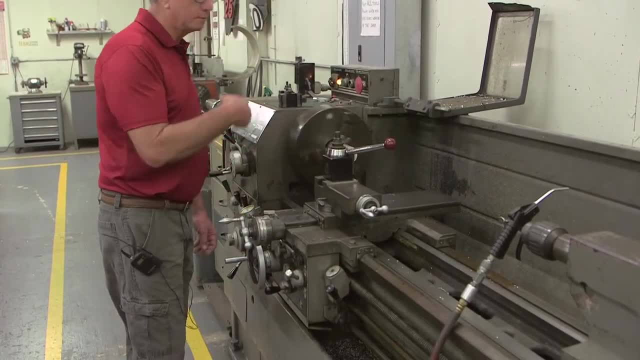 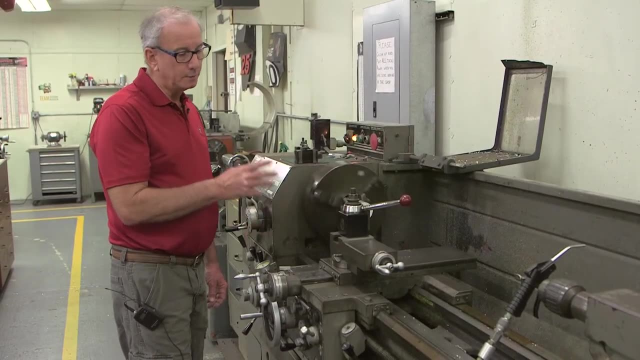 We can also pull it upward and it'll rotate in the opposite direction. This is the way we do not want it to be turned on. If we do this- and we've had students do this- it ruins their parts and makes a mess. 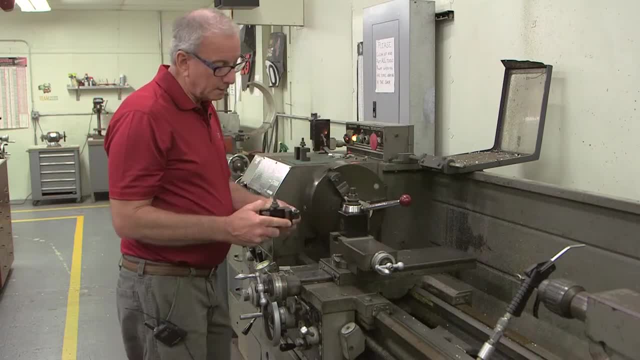 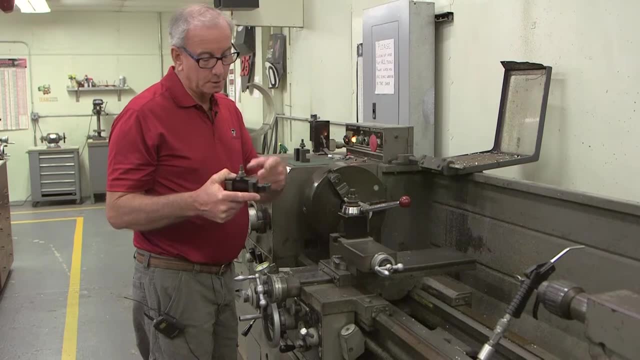 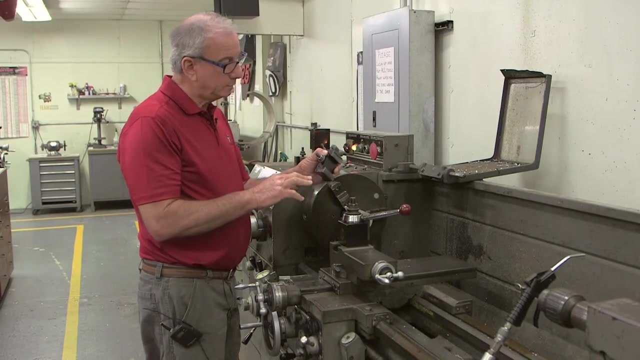 It's hard on the machine. The cutters are like this: They mount in the tool post and the rotating part comes down against the cutter, so it needs to rotate in the correct direction. All of our I've labeled This tool post. 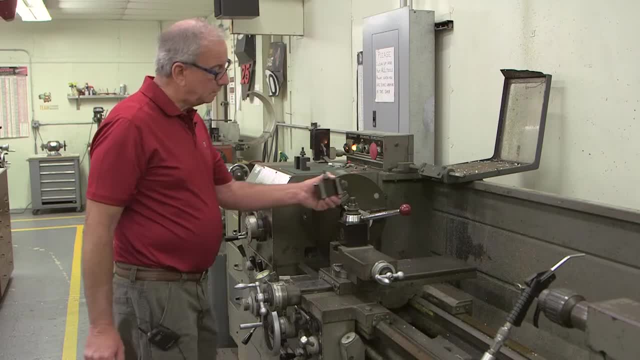 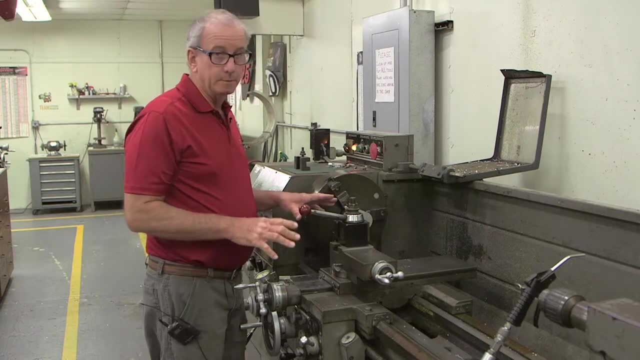 This tool post's sharp to be for the sharp machine. You put it in the tool post, clamp it down. and the reason why it says sharp and it's labeled for this machine is the tool is right at the center line of the part. 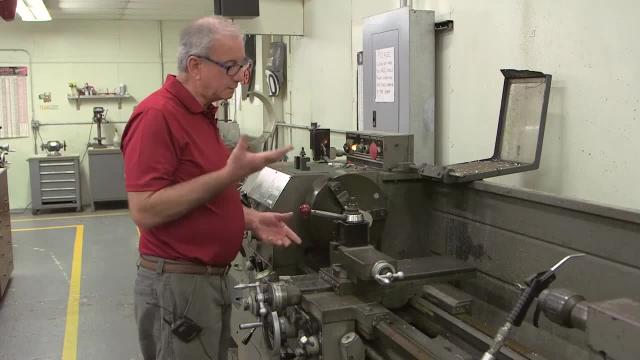 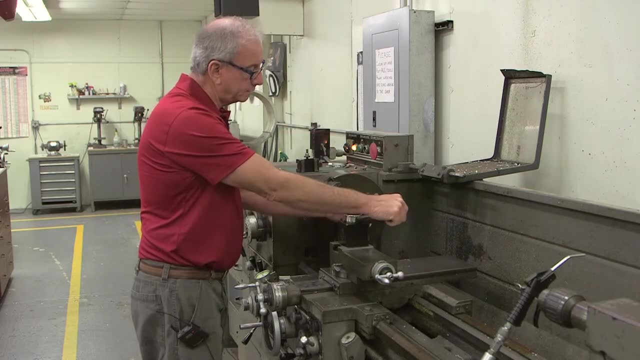 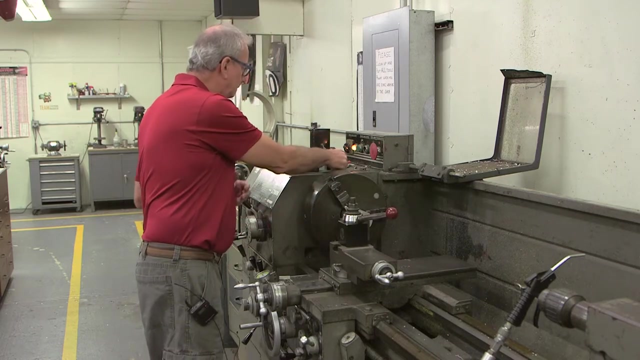 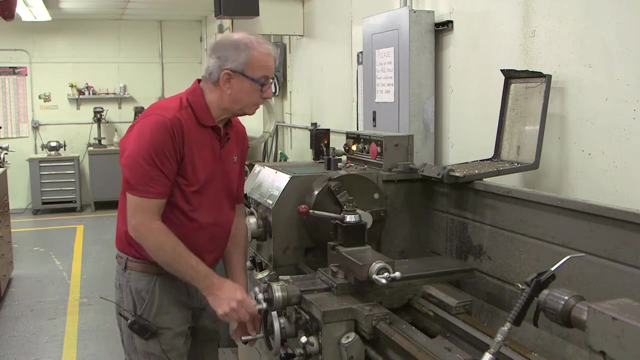 So the tools, whatever tools you use, need to be set at the center line of the part. This is a form tool, Does the same thing. It puts a nice, It's a nice 45 degree chamfer on your part. This tool is a normal turning tool. 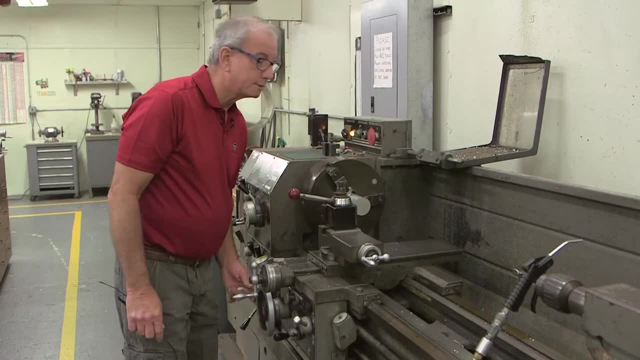 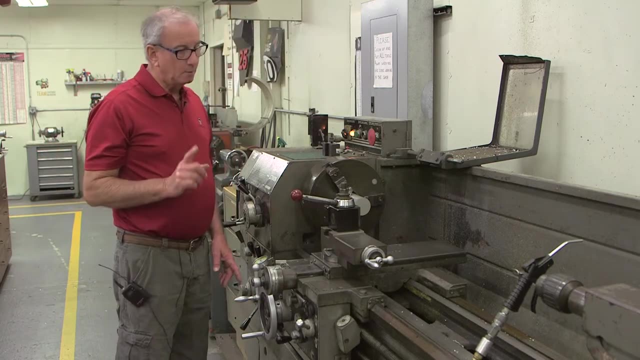 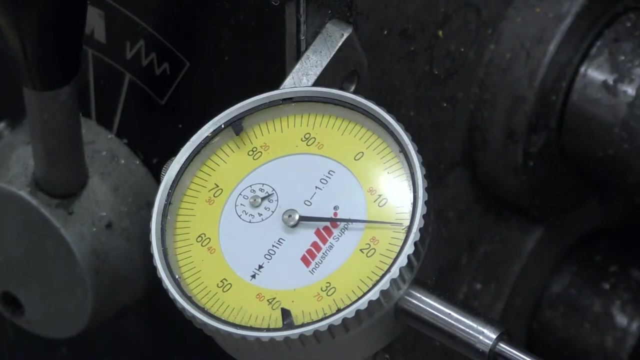 It will face off and also turn your outside diameter. It provides two separate functions. One of the things that I've installed in this shop two summers ago is a travel indicator. What we'll use the travel indicator for is that we can bump up against our face. 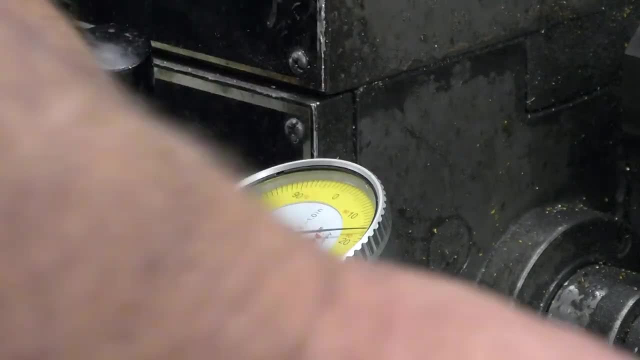 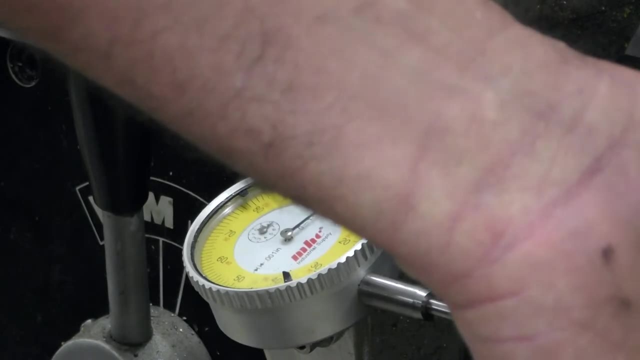 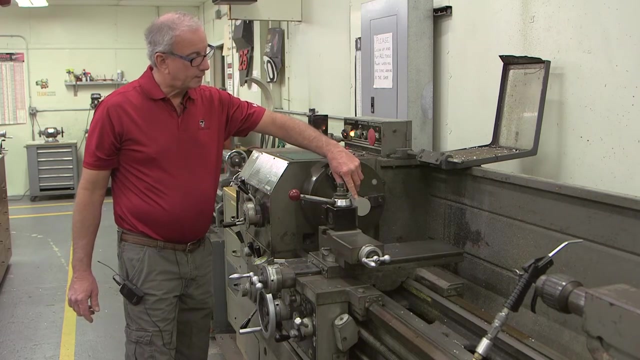 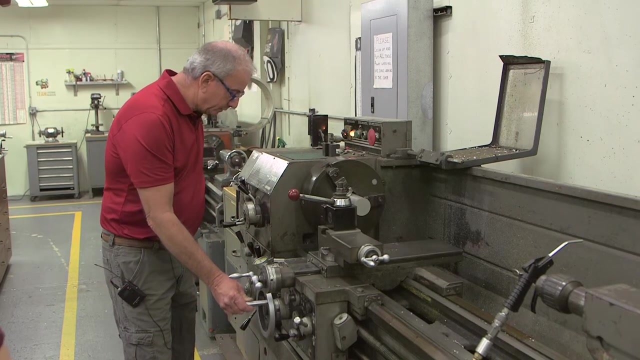 This is the face of the part. We can zero our travel indicator And then we Say we want to come back 500 thousandths and turn a shoulder here, so we can take our travel indicator And go one, two, three, four and 500 thousandths.